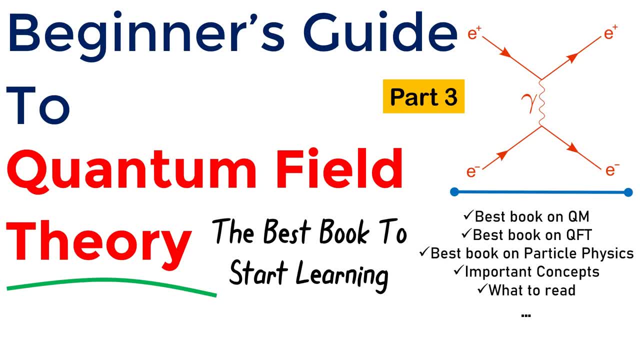 Books that I believe are absolute must-haves for anyone looking to explore these topics. These books are not only informative, but also written in a fashion that is very friendly for any beginner. My name is Sean Ack and you are watching this video on my channel, Physics for Students. 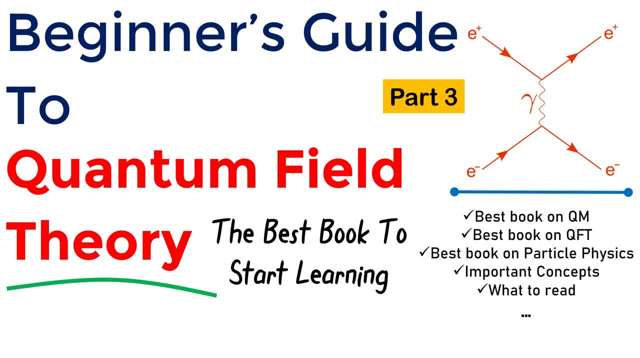 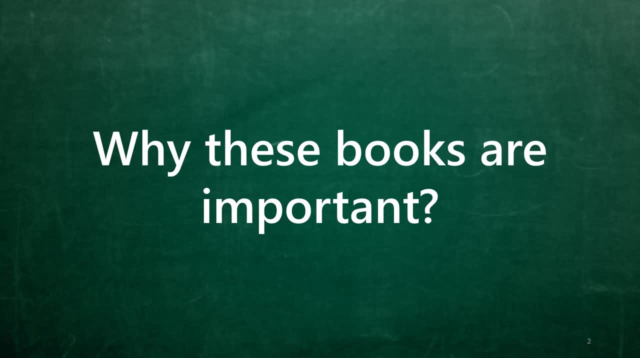 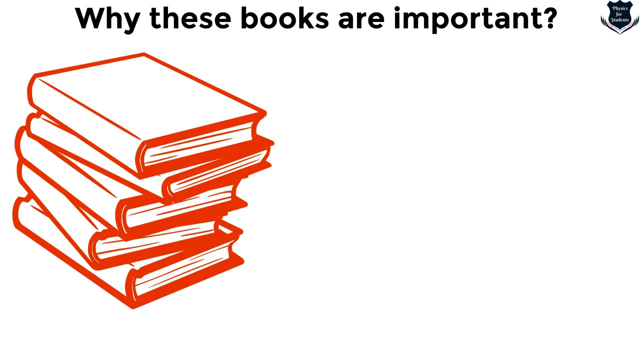 Welcome to the third episode, where we are exploring how to learn quantum field theory, And this video will be essentially dedicated into learning methods and what are the best methods. So first let us understand that: why these books are important. Now you see, these books are like portals to the minds of brilliant physicists and scientists who have really spent years and years unraveling the mysteries of the universe. 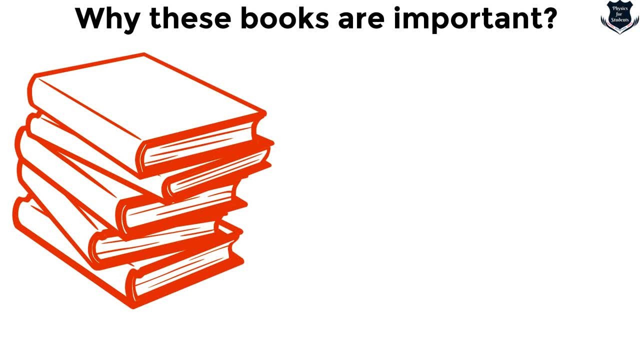 They contain the distilled wisdom of generations, the key to understand the building blocks of reality and the gateway to grasping the most profound concepts in science. So, number one, These books are important. These are the best books for beginners in quantum mechanics, particle physics and the ancillary areas of quantum field theory. 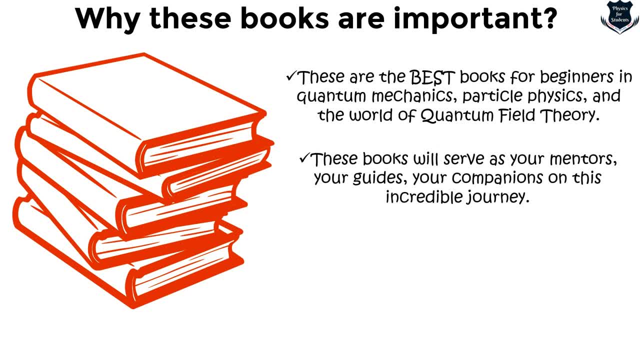 These books will serve not only as a book, but, I would say, as a mentor or your guide or your companion on this incredible journey, And whether if you are a complete newcomer or you have already started learning the subject of quantum field theory, or if you are looking to deepen your understanding what you have already learnt. 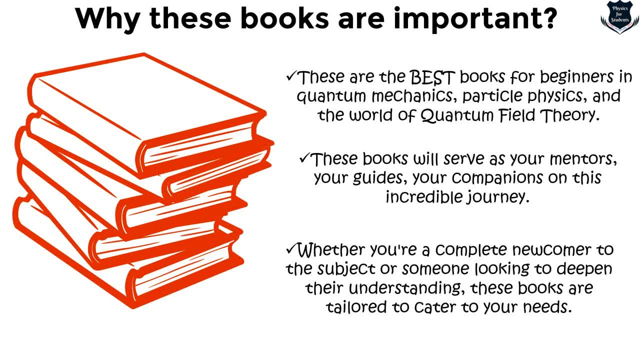 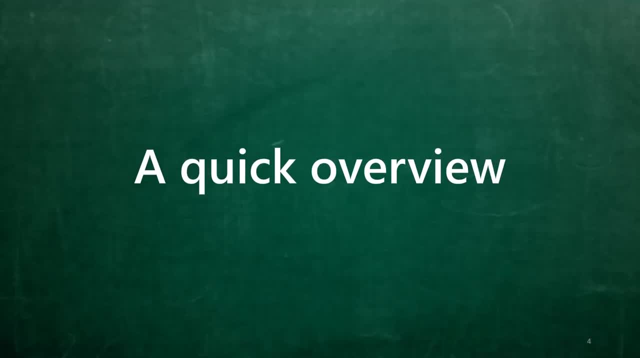 then these books are tailor-made and this will cater to you. So, having said this, that these are the most important factors, and that is why we need the books, First, I would like to give you a quick review of those who have missed my first and second episodes on learning quantum field theory. just quickly, so that you won't miss on the important concepts. 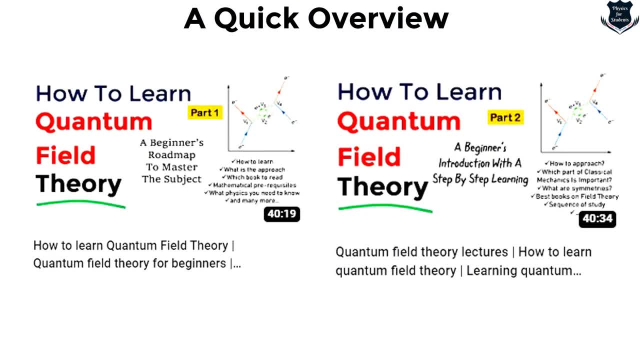 So here you see, I am showing you the thumbnail, part one and part two: how to learn quantum field theory. It is there in my channel physics for students. You can just quickly go there. As you can see, these are almost more than 40 minutes because I have divided these into blocks and then sub-blocks, and then the mathematics, then the physics. 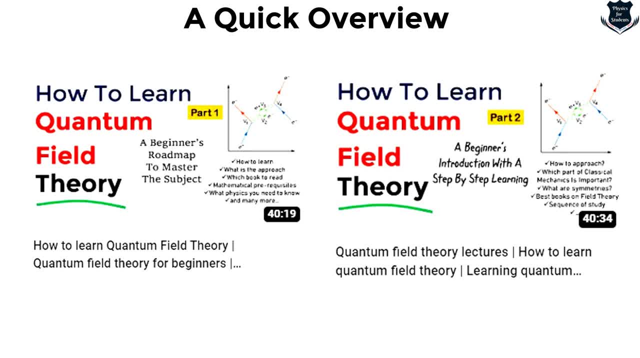 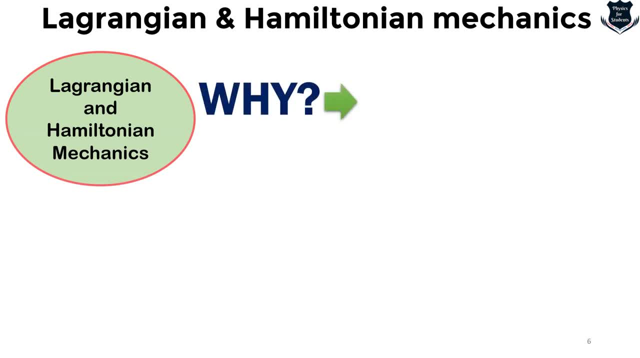 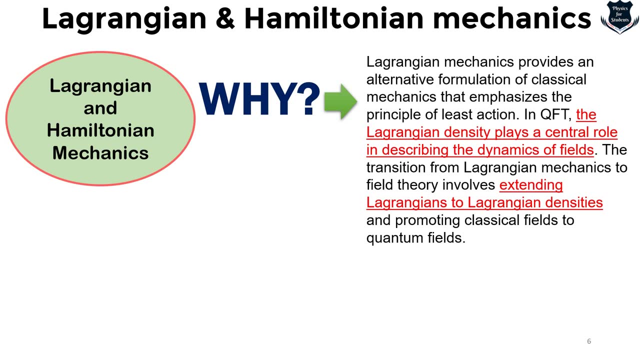 What are the books, What is the sequence? So you can go ahead with that. First is that what we have learnt earlier is this one. We have learnt that why do we need Lagrangian and Hamiltonian mechanics? And we have said that in quantum field theory, Lagrangian density actually plays an important role because from particles we are moving forward. 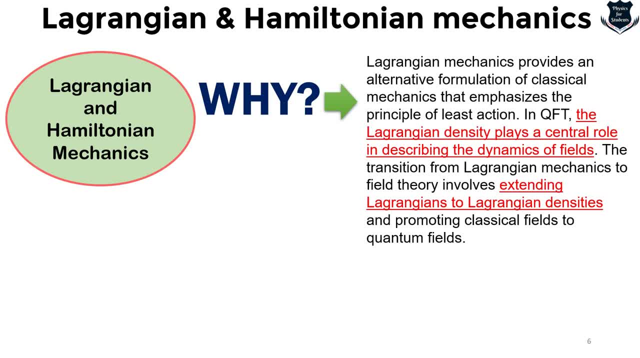 We are moving into fields and this field theory actually extends Lagrangian to Lagrangian densities. Right below you, as you can see, this is the Lagrangian equation, which is further, you know, have been used double integration in order to sum up the density. 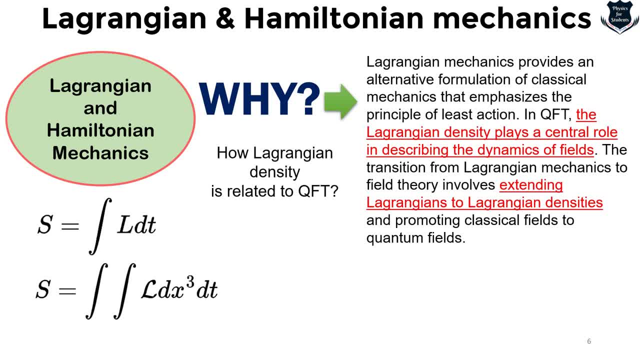 So how Lagrangian density is related to quantum field theory. it is there in my second video which you can watch, But this is the basic summation that the Lagrangian density measures the distribution of the Lagrangian density, Which is the distribution of the Lagrangian space, of the Lagrangian over the Lagrangian space. 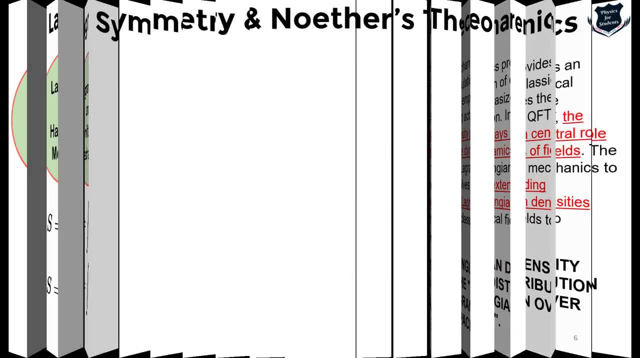 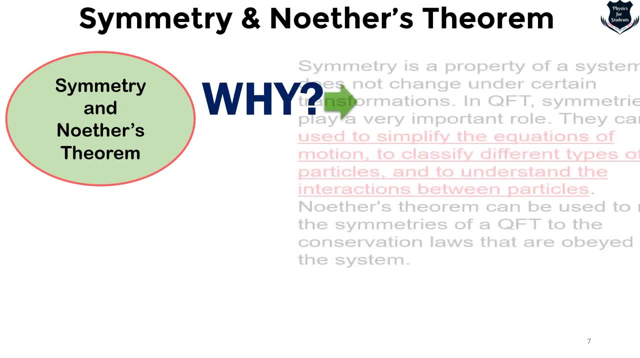 So if you want to know more about that, go to the second video, which contains these details. We have also, you know, looked into what is called symmetry and Noether's theorem, And we have seen that these are used to simplify the equations of motion to classify different types of particles. 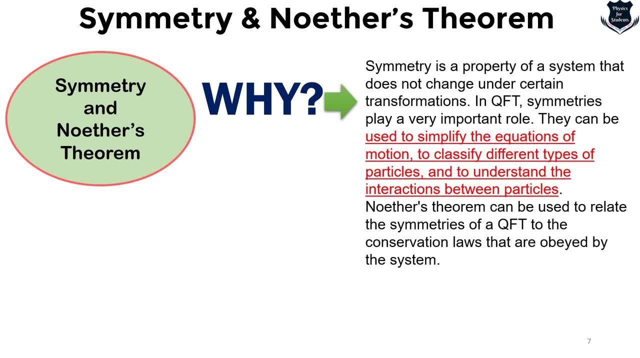 And Noether's theorem is actually a very significant contribution, And it is used in many ways to relate With the symmetries of quantum field theory. We have also seen that symmetries provide a framework in order to understand how physical quantities actually behave and transform. 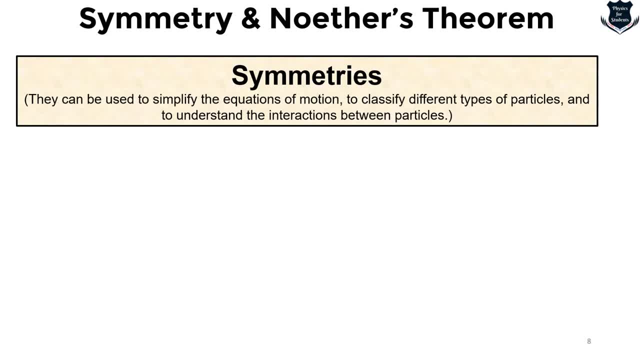 And what are these the symmetries? we have earlier looked at it, So I won't go into much details. We have seen what are continuous symmetries, translation, rotational and Lorentz symmetries, discrete symmetries: We have seen internal symmetries, including isospin, flavor and chirality. 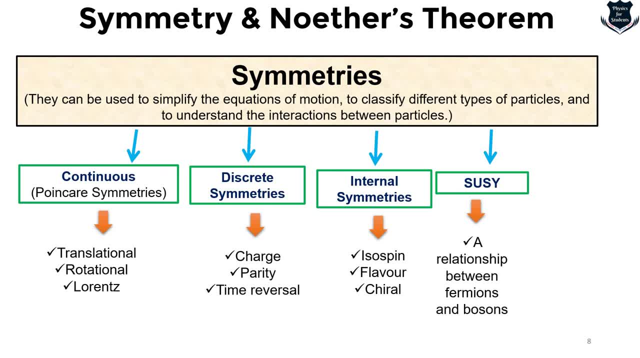 We have seen the famous SUSI, that is, the symmetry. Symmetry is relationship between fermions and bosons, And we have also seen what is called a conformal symmetry. Now, very recently, I have made a video on what is called the Noether's theorem. 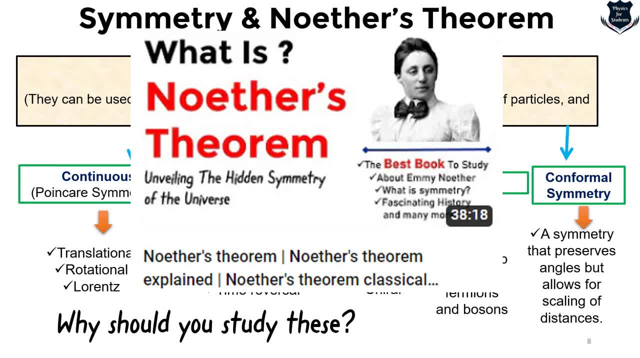 And I think that if you go ahead and check onto it, then you will find much more details about Noether's theorem. Only yesterday I have launched that video. It contains the details of Noether's theorem, each and every symmetries, Not only how Noether's theorem actually saved Einstein, David Hedbert and Felix Klein from generativity which seemed to be violating the law of conservation of energy. 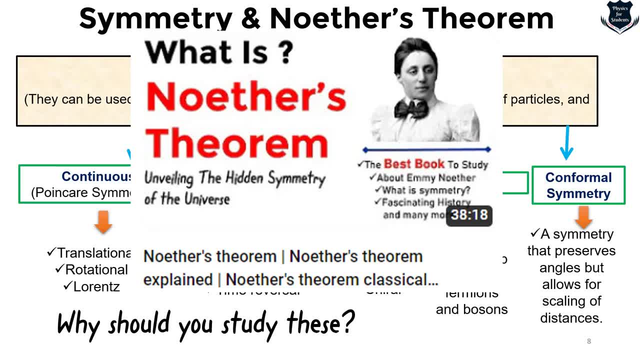 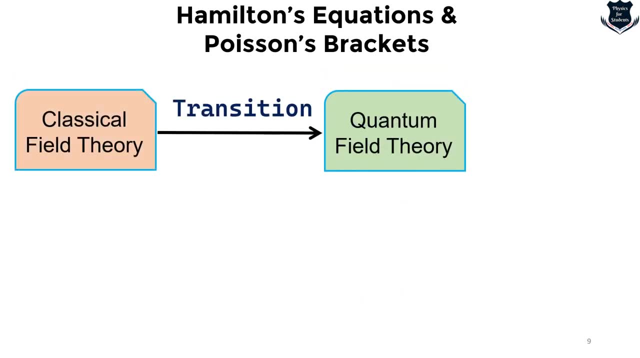 So this is one of the most beautiful, I would say, theorem in physics. So if you are really interested, other than quantum field theory, here is the video Noether's theorem unveiling the hidden symmetry of the universe. You can go ahead and check it. We have also dealt with Hamilton's equations and Poisson brackets, which is actually a transition. 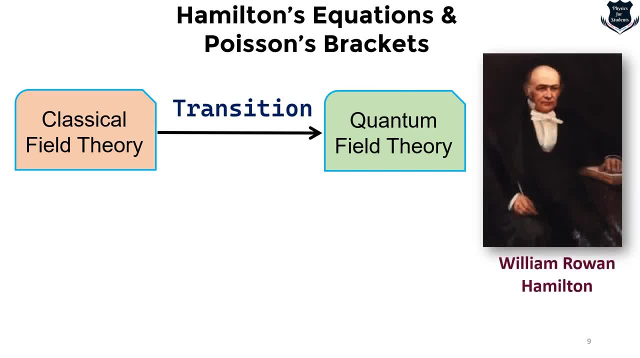 What we call, from classical field theory to quantum field theory, And I have, you know, described in details what are Poisson brackets. So these are again in the second part of the video and you can go ahead and find it out. Classical fields to quantum field operators, what are the things? 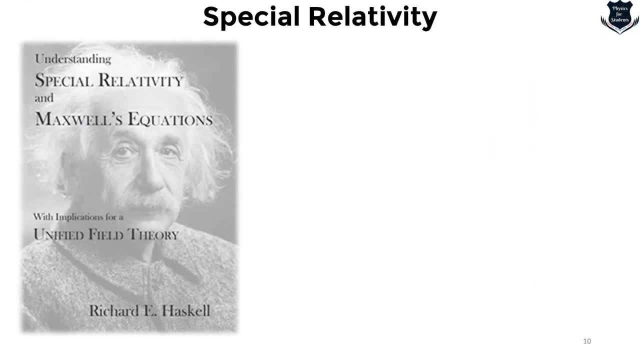 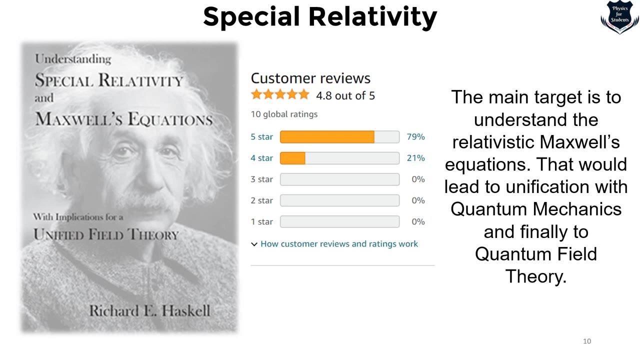 And, most importantly, Dirac's canonization equation. that is called quantization, or I would say canonical quantization. We have also looked into why do we need to understand this book, That is, our special relativity, taking into consideration Maxwell's equation, because relativistic Maxwell's equations are the stepping stone for the quantum field theory. 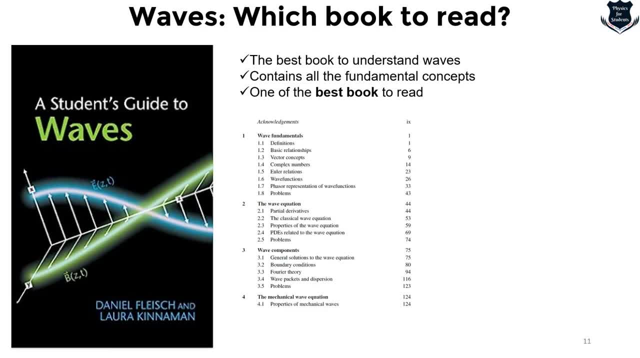 I have also given an understanding of this wonderful book by Daniel Fleisch and Laura Kinman, which is called a student's guide to waves. And these are the basic, because quantum mechanics and further quantum field theory is based on wave mechanics. So until you know what are waves, wave equation, wave components, electromagnetic wave- it won't be possible. 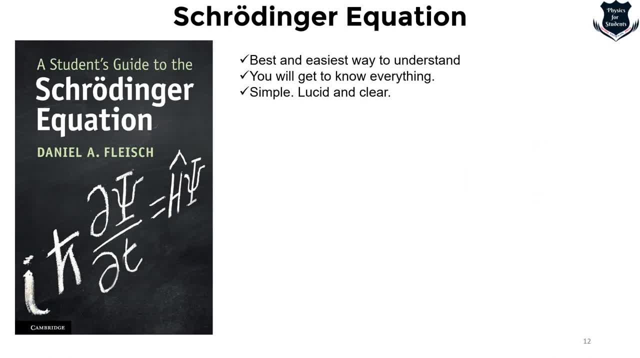 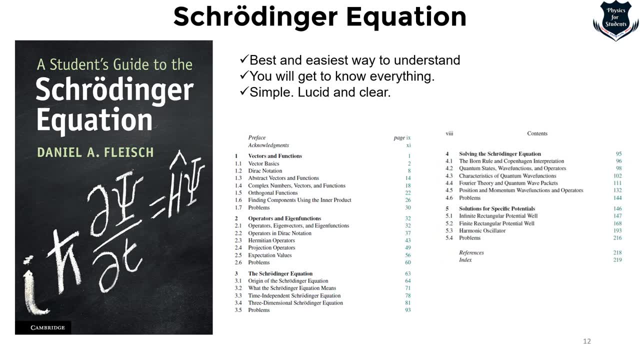 And this is one of the best book That I would suggest. also, I have spoken a lot about this book, which is called Schrodinger equation by Daniel Fleisch, And this gives a detailed understanding of Schrodinger equation. And, most importantly, this book assumes nothing and builds up right from the basis, including vector functions, Dirac notation, eigen function, projection operators and so on. 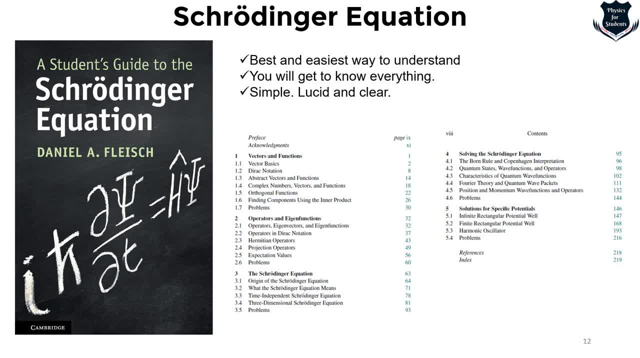 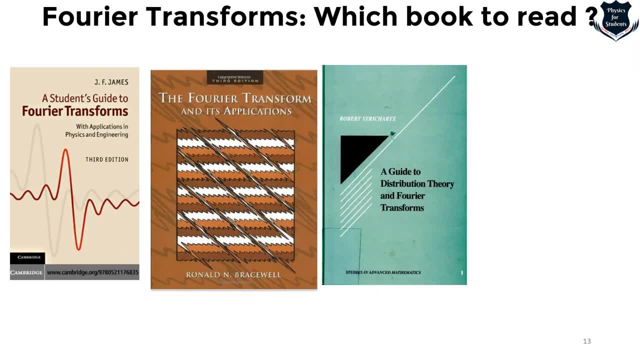 So these are the books which we have talked in details And, most importantly, there are certain books on Fourier transformation. So these are the four books which I have suggested. out of that, This is the first book you need to read, This is the second. 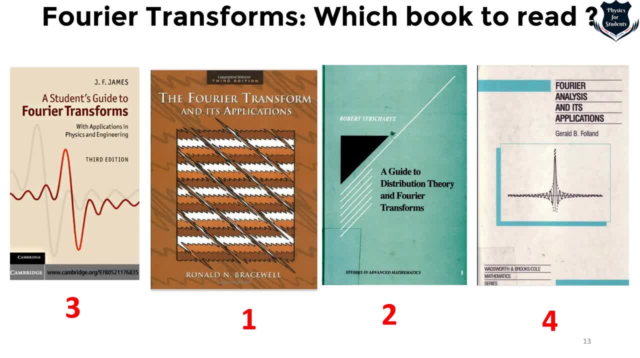 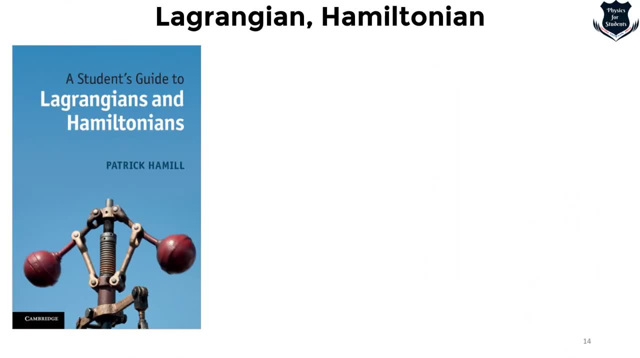 This is the third and the fourth. However, all these four books of Fourier transform are equally important, But if you go sequentially I think it will be very easier. Lagrangian and Hamiltonian are utmost important. This book of Patrick Hamill is very important in terms of Lagrangian Hamiltonians. 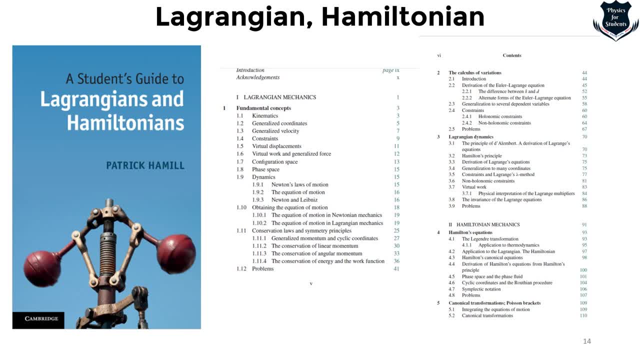 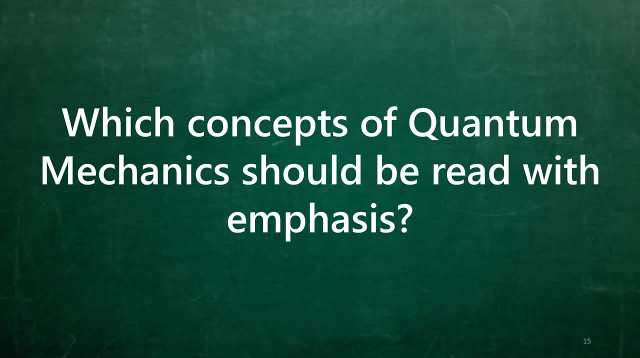 And I have given quite a number of details about Lagrangian Hamiltonian. This is very important. This is very important. This is a very good book to read with Now. apart from this, what we need to understand is that when we go further into learning quantum field theory, what is important is quantum mechanics. 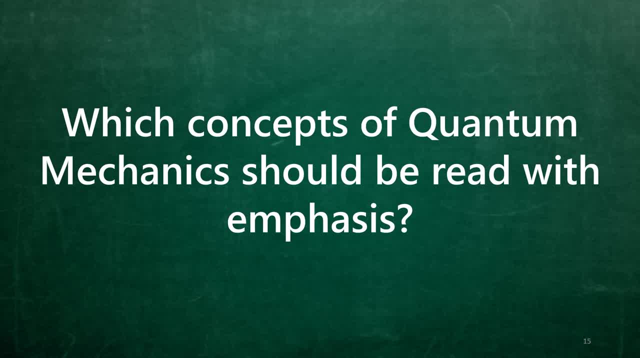 So, at the core of framework of the principles of quantum field theory is quantum mechanics. We can call it as, like, the Rosetta Stone of the universe, allowing us to decipher the language of particles and forces. Now, out of the many books, Innumerable books of quantum mechanics which are available online, 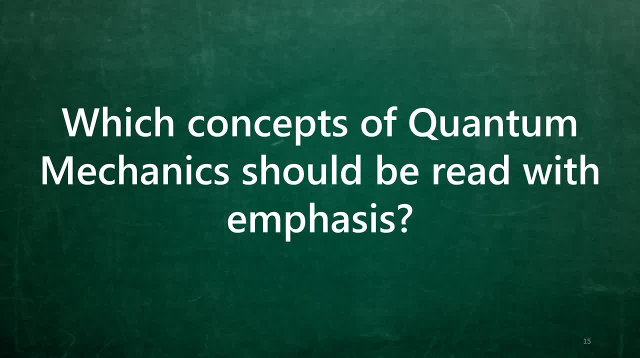 Lecture notes, Hard copy books. I have listed down few of the books which are very important. Now, before going ahead dealing with the books of quantum mechanics, I would like to tell you that what are the concepts of quantum mechanics which you specially need to emphasize and learn? 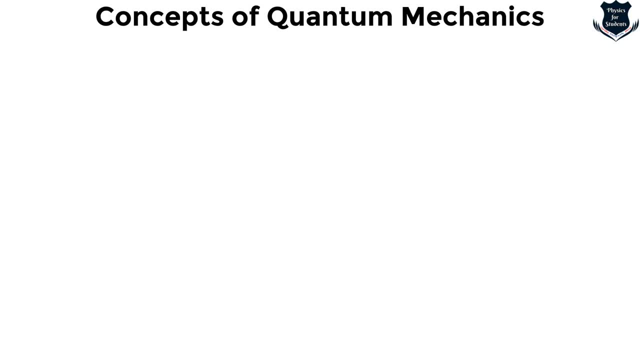 Because you are keeping into mind the long term target, that is, learning quantum field theory. So these are the things which you are learning- quantum mechanics as a whole- in the course, But these are the concepts which you must learn with much more emphasis. First is the wave particle duality. obviously, because this is the basic paradigm shift in terms of mental and fundamental mathematics. 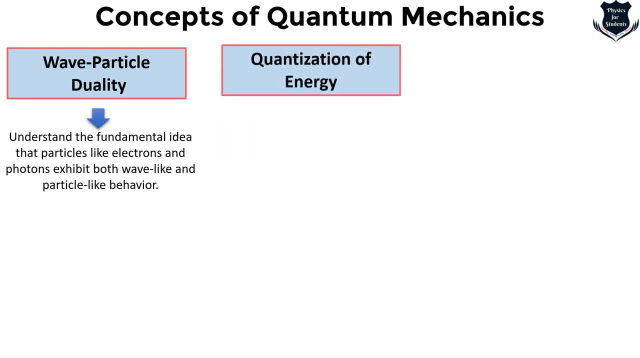 That electrons and photons behave both wave life and particle like behavior. This is important. quantization of energy, because this is again a fundamental stepping stone from the continuous. Now we move into quantization of energy, You also need to learn about what is called wave function. 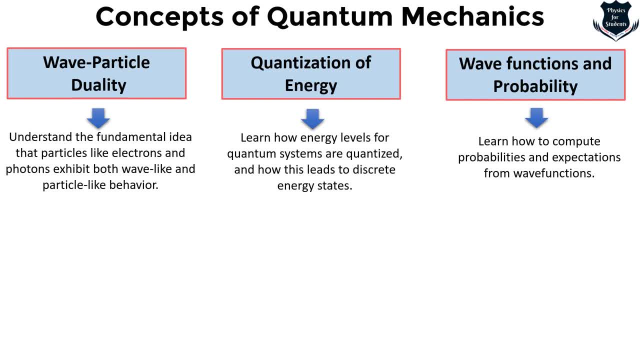 Wave function and probability and better to do a lot of mathematics into calculating wave functions using the bra and ket notation and the probability part. This is again important Operators and observables, Because in the last quantum field theory, part 2, I have shown you that what is called canonical quantization is that the basic observables of the classical mechanics are now being replaced by operators in quantum mechanics. 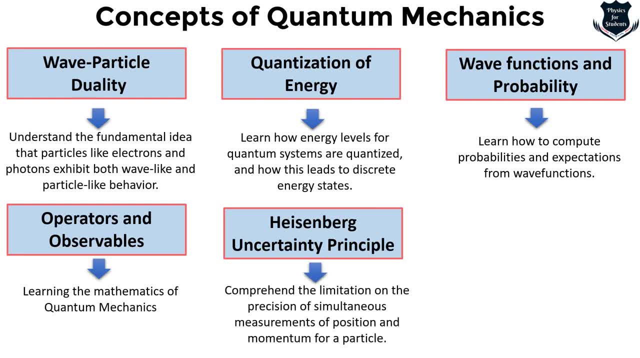 So this is also important. I think I don't need to explain this famous principle, Heisenberg's uncertainty principle. I would recommend go back to one of my videos where I have taken a deep, deep dive into understanding Heisenberg's principle from Fourier transform. 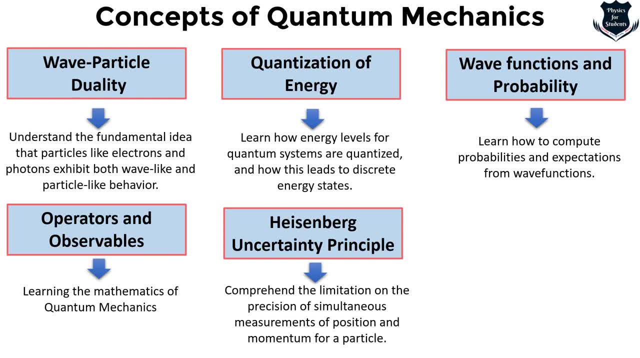 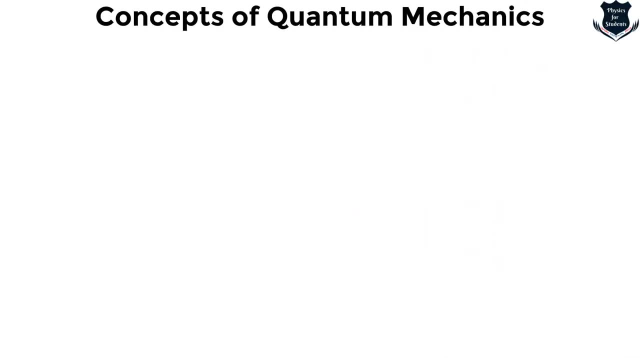 And what are the similarities and why you should understand Fourier transform in order to understand Heisenberg's uncertainty principle, The both time dependent and time independent equations of Schrodinger equation. This is important. You can refer to the earlier book which speaks very easily about Schrodinger equation. 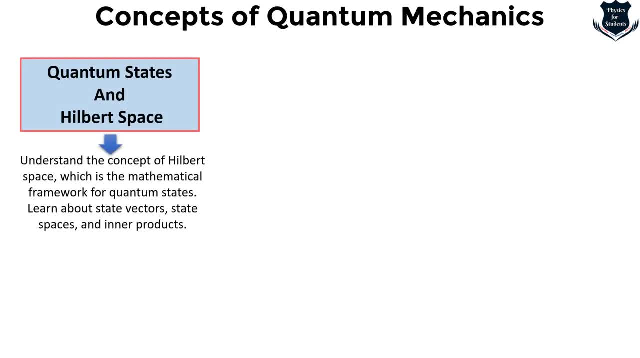 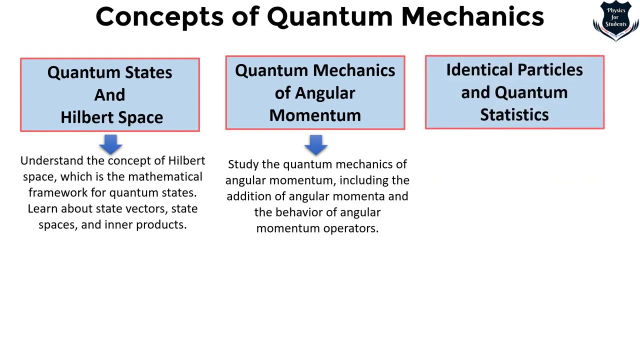 Quantum states and Hilbert space. Well, this is something a little bit more mathematical. You can go back to my video on the mathematics of quantum mechanics, which I would take 3-4 more videos to complete the entire playlist. You need to learn a lot about angular momenta, because the angular momentum operators are dependent on this. 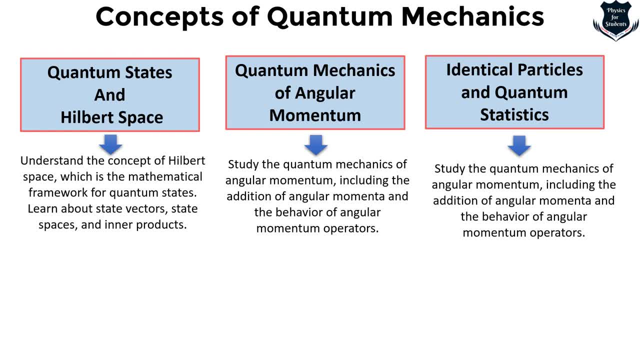 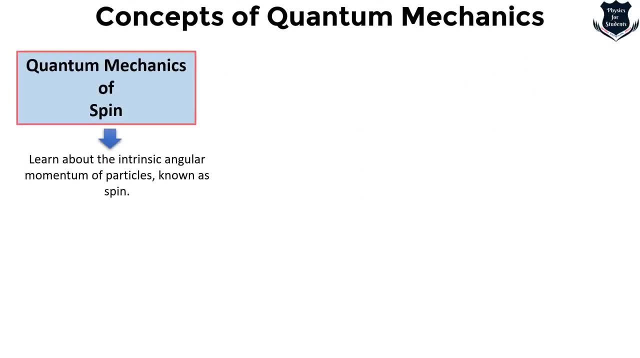 Identical particles and quantum statistics- This is also important- Including the addition of angular momenta and angular operators. You also need to learn a little bit about quantum mechanics, The spin, How the particles behave, The spin of the particles, etc. And the approximation methods. 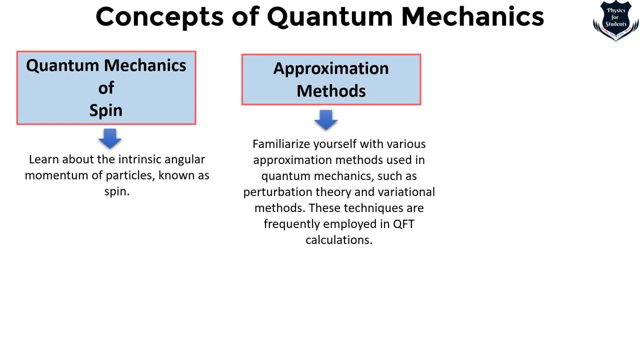 Approximation methods are important because in perturbation theory, especially in quantum mechanics, what we do is that we give a lot of emphasis on approximation methods. So these are the concepts I would say, apart from the entire understanding of quantum mechanics. I would suggest strongly that these concepts should be read, understood. 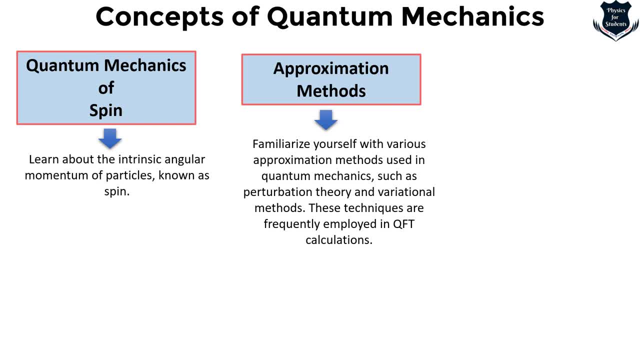 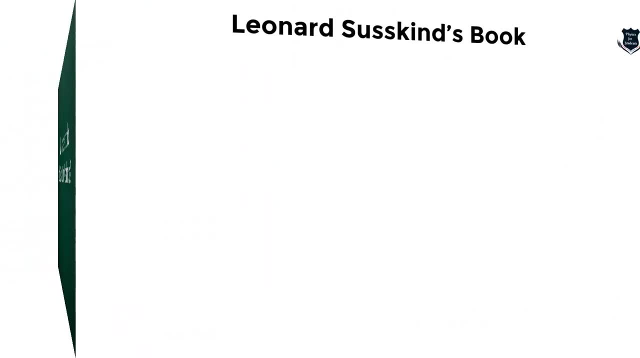 You can do a lot of examples on that, because based on this, you are again moving into quantum field theory. Coming back, What are the best books of quantum mechanics? First of all, I would like to recommend Leonard Susskind's Quantum Mechanics of Theoretical Minimum. 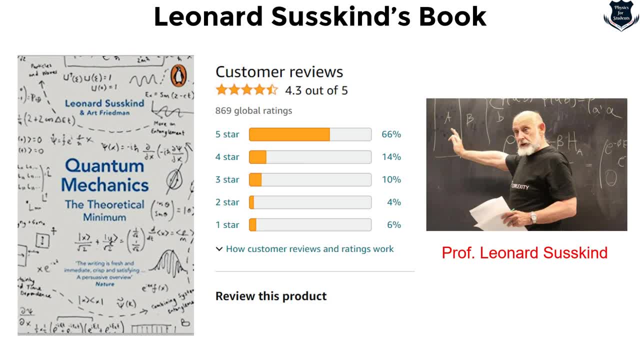 This is an absolutely amazing book and I can tell you with a lot of responsibility, that if you go through the entire book, You really don't need any other book to read. But however, different books give different kinds of details, so it is better to consult more than one book. 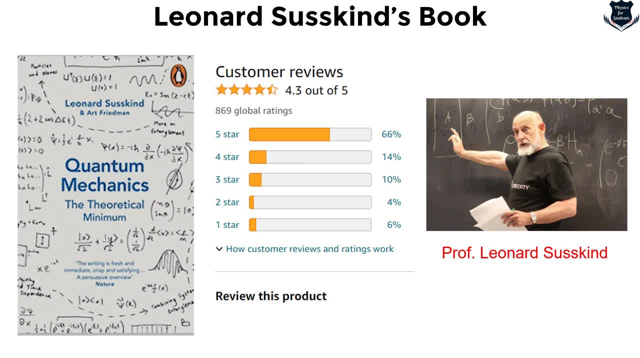 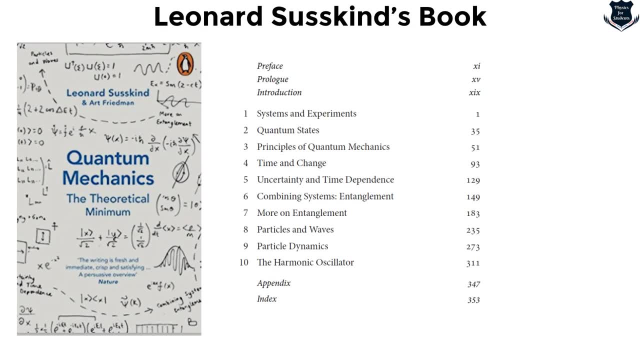 So you can see already it is 66% which is showing customer review in Amazon, which is called a 5 star. Now this book, if I go for the basic content part. So these are divided into 10 lectures, starting from systems and experiments. 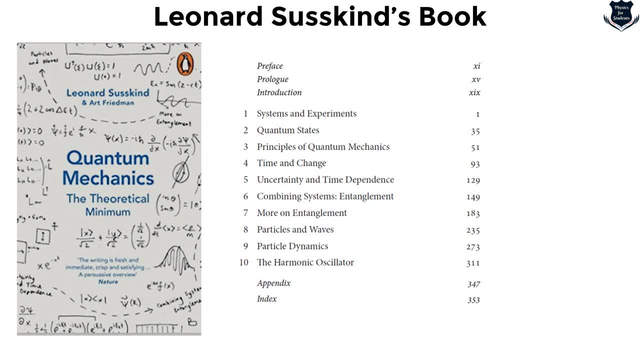 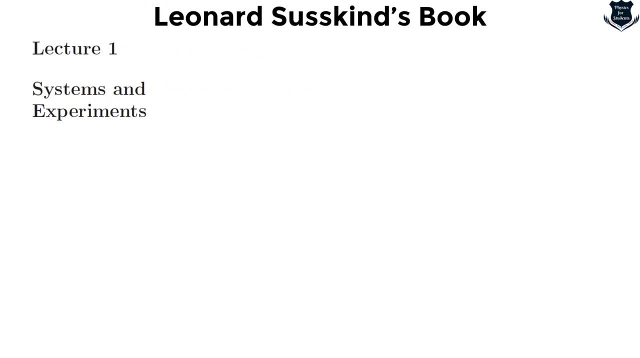 Now why I am telling that this book is the ultimate book and really you do not need any other book. I will soon justify So. you see, the first lecture starts with systems and experiments, Which very less number of book actually shows you that what are the system and what are the experiments? 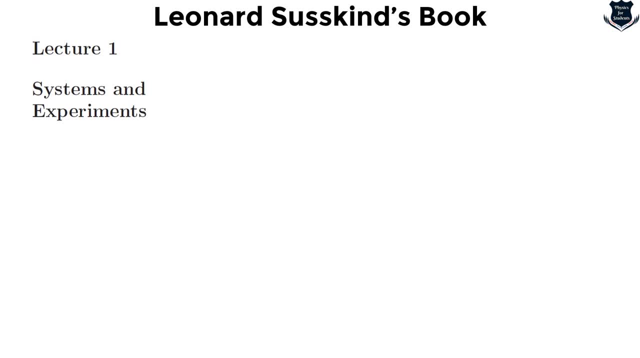 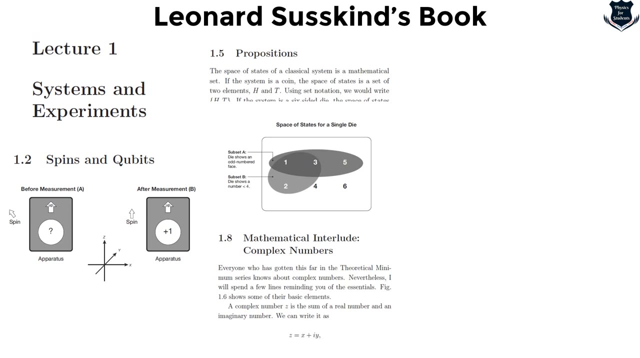 And these experiments results produce something which we called counter intuitive, and things starts to mature. So it starts with spins and qubits and you can see there are nice diagrams using single die, how the spaces of states, And this is absolutely amazing. Most importantly, 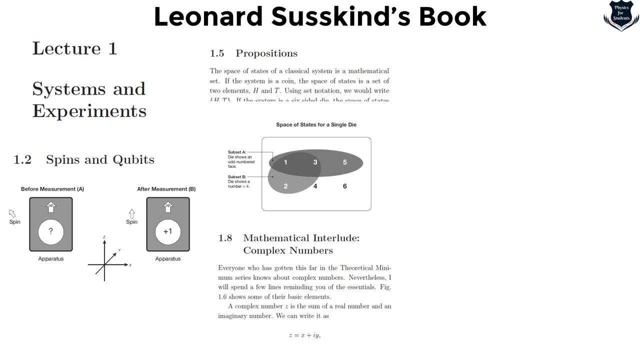 Professor Leonard Susskind. what he has done is that in between, if you need a mathematics, he has included that Mathematical interlude like complex numbers. Then there are functions, vector spaces, everything- Whatever you need that you don't know. the mathematics in between, he will take a pause and go ahead. 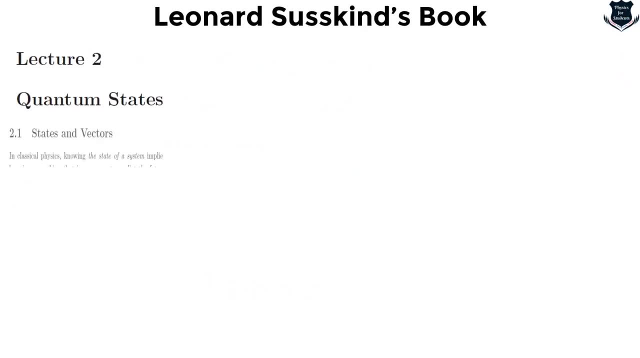 Brass and cats, inner products, etc. Lecture 2 starts with different kinds of quantum states, including state vectors, spin states, column vectors. Absolutely, this is easy, anyone can understand. Again, a mathematical interlude, Because you need to know the machine matrices. 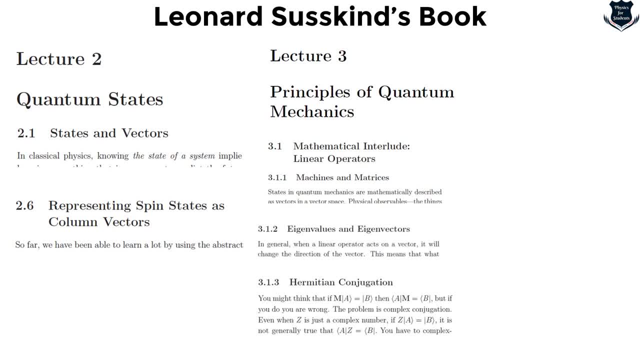 The Eigen values, Eigen vectors, Hermitian conjugation, So wherever you need it. there is a pause and he is going back making you understand the mathematics and going ahead with the lecture. So you see the Gram Schmidt procedure constructing spin operators and spin polarization principle. 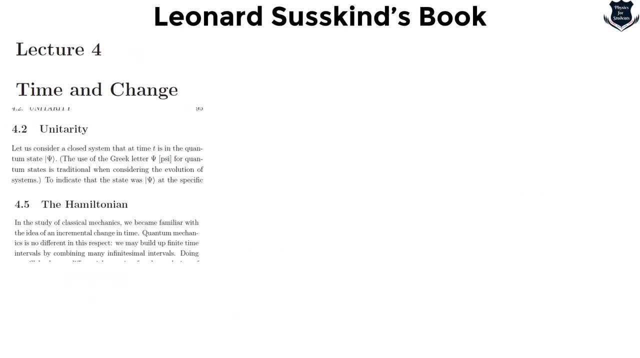 The lecture 4 starts with time and change, which includes unitarity, The Hamiltonian. what has happened to H bar? that is, the reduced Planck's constant, The conservation of energy, the collapse of the wave function. Lecture 5 starts with uncertainty and time dependence. 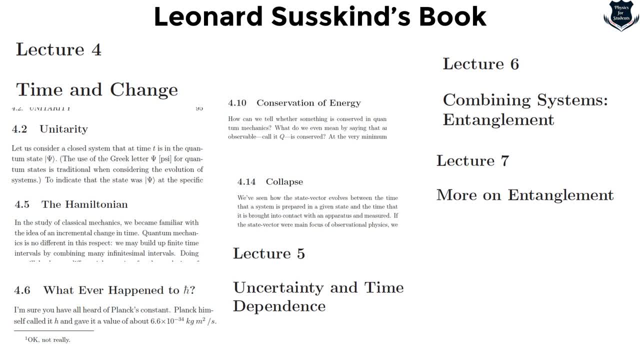 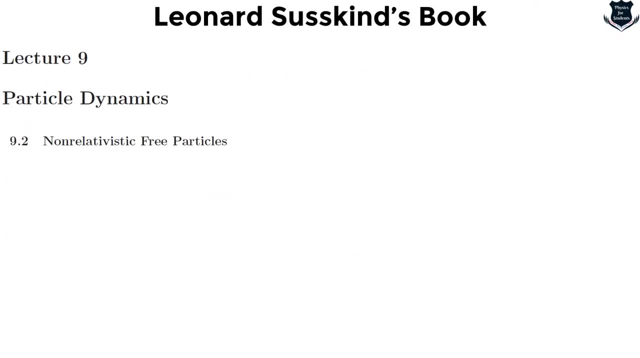 I am not going too much because it is a 350 plus pages book. The entire video will be consuming this time. So lecture 7 is on combining system. more on entanglement, particles and waves. Lecture 9 specifies on particle dynamics, which starts with non relativistic free particles. 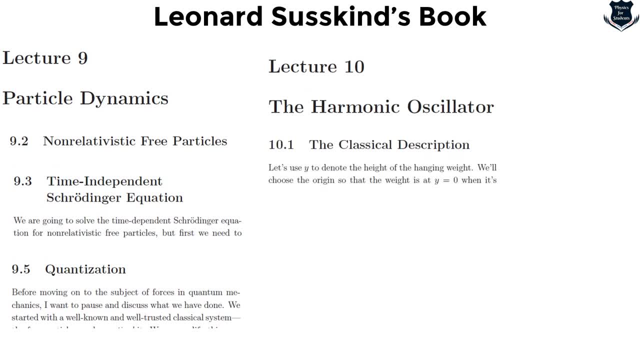 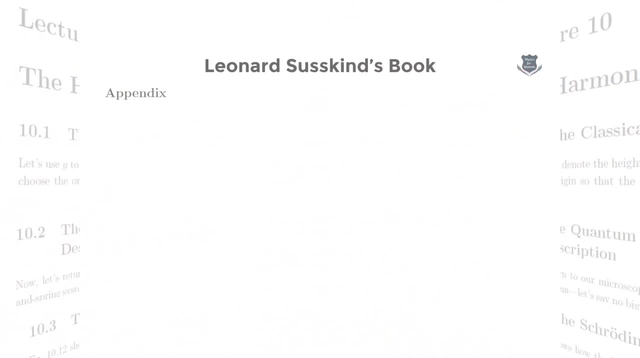 And then the time independent Schrodinger equation. It deals much more details in what is called a quantization, Gives several other examples which would be absolutely great if you read it. Lecture 10 starts with the harmonic oscillator, classical description, quantum mechanical description and the Schrodinger equation. 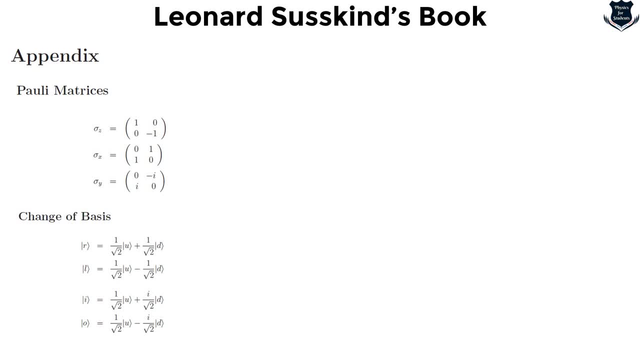 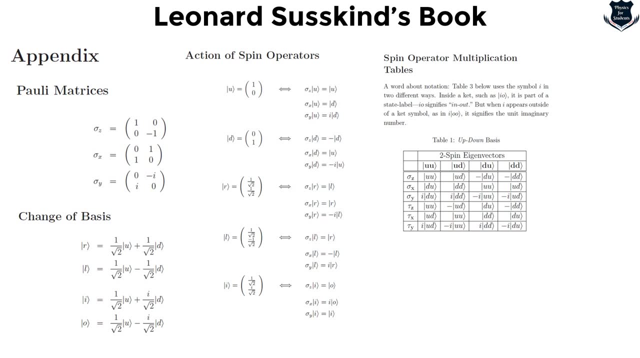 So even you can see the appendix- it is such beautifully organized- The Pauli matrices, the change of bases, action of spin operators, Even the table that he has used that is the spin operator, Different types of operators using spin operators, Different eigenvectors. 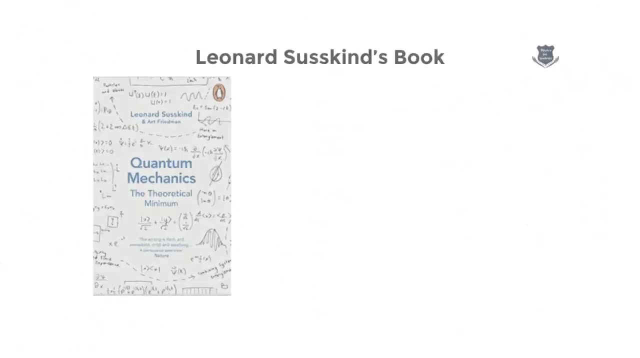 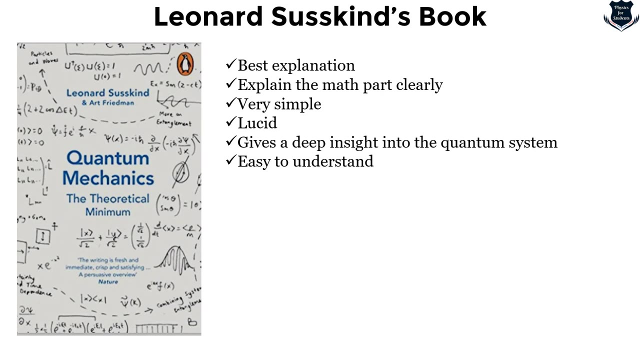 All these things are included. So what I can tell you at the end is that this is an absolutely best explained. The math part is clear, Very simple, lucid, Gives a very deep insight and it is very easy to understand. So classical and quantum: the difference is very clearly and deeply philosophically laid out. 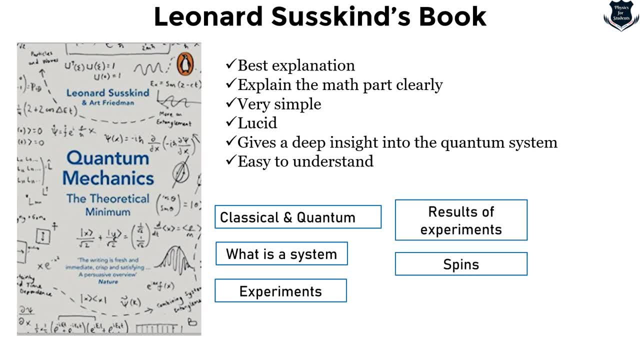 What is a system: experiments, results of experiments, spins and vector spaces. So all the mathematics is included, The physics is included And wherever you need to go back and understand the mathematics, He has taken an interlude kind of a thing and he has gone back and he has made it clear. 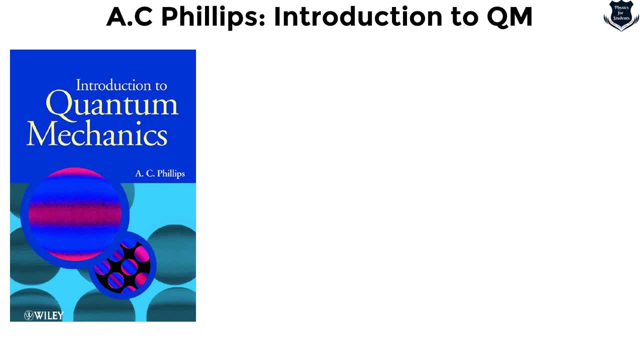 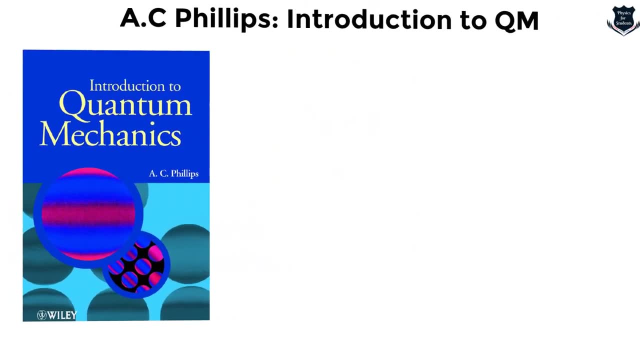 The second book I would recommend is very good for beginners. That is A C Phillips introduction to quantum mechanics. Already you can see 66% votes for a 5 star and I would like to show you quickly the table of contents. So you see it starts with Planck's constant inaction. 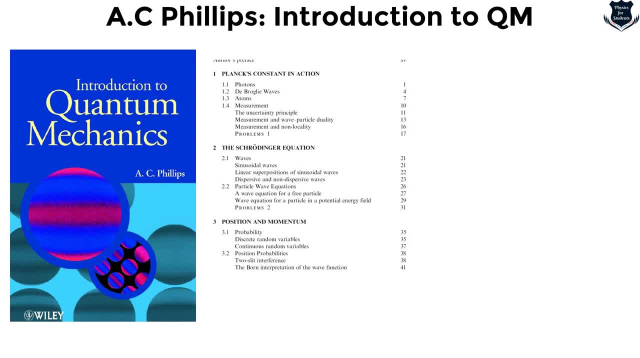 Then it goes to Schrodinger equation And very easily described. I mean to say, if you read this book you will understand Position and momentum, Energy and time, And then it goes into square. well, That is the quantum barriers Harmonic oscillator. 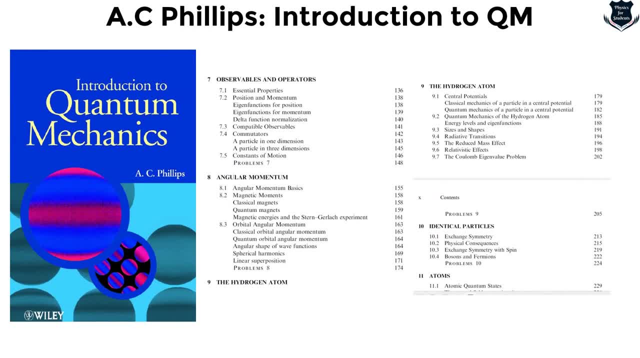 Further. the books also lucidly explains what are called observables and operators, Angular momentum, And he takes the example of a hydrogen atom, which is relatively easy to expand on the mathematics He uses the relativistic part, Identical particles, atoms and so on. 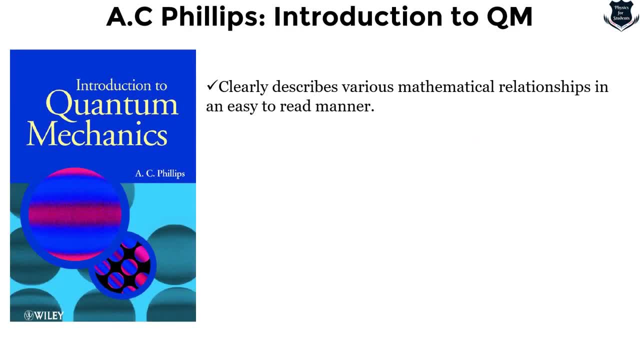 So what I can tell you in a nutshell is that this book clearly describes various mathematical relationships. It is absolutely easy to understand. This book requires just a little bit of knowledge of calculus and the classical physics that you need to know, And it explains clearly with appropriate amount of maths. 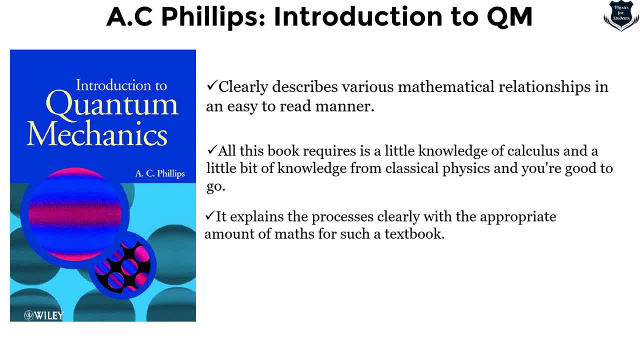 That means not much of mathematics is concerned, Not less of mathematics is concerned. It is absolutely appropriate And the quality of writing is basically to encourage And stimulate the undergraduate student encountering these topics for the first time. So if you are an undergraduate student, 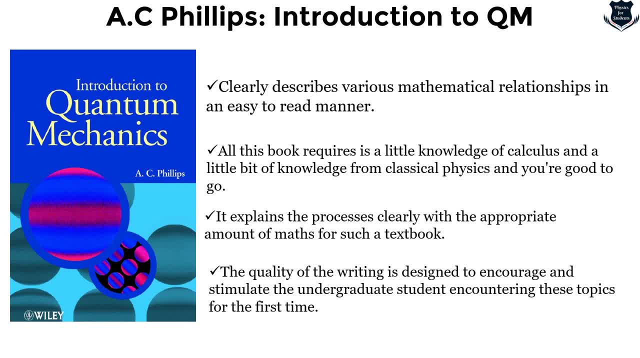 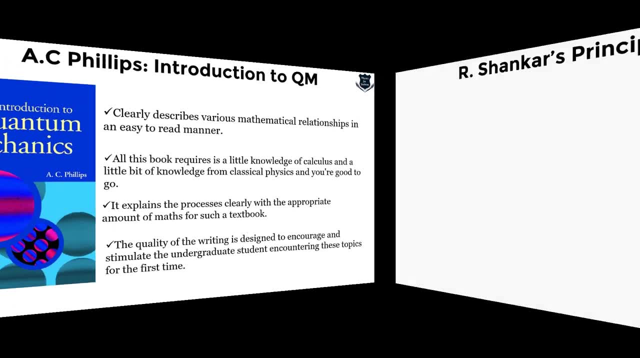 If you are encountering it for the first time, Then this book would be absolutely an amazing book for you. So this would be a second recommendation. AC Phillips: introduction to quantum mechanics. Now, this book is absolutely great. I mean to say this is by a great person called R Shankar. 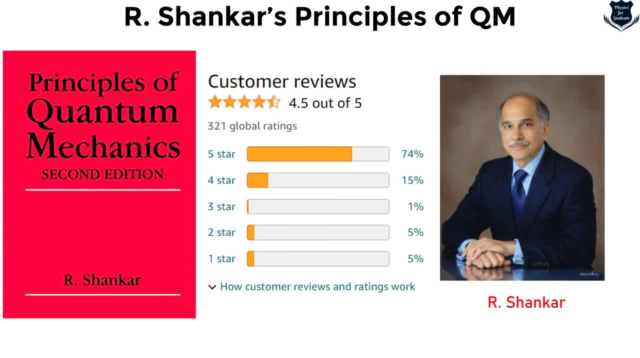 I think everybody knows about Professor R Shankar. This has already got a 74% rating. A 5 star Principles of quantum mechanics, Although the book seems to be a little bit more mathematical. But this book starts from right, from the beginning. 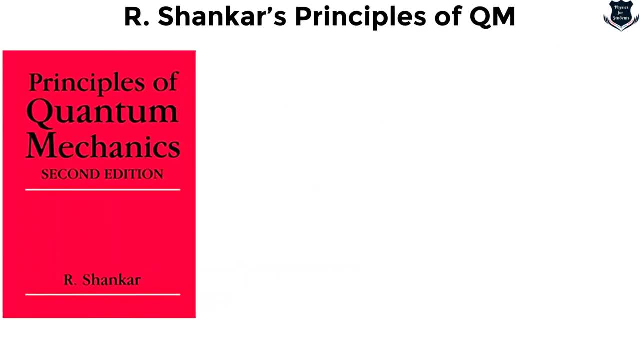 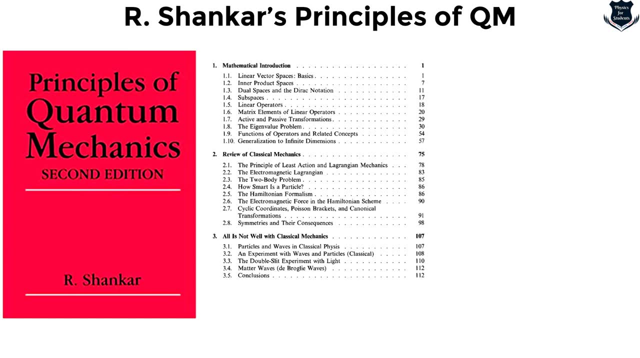 And it shapes in a very nice way. Let me show you table of contents of this book. So you see, it starts with the mathematics, Mathematical introduction, Which is again quite beautiful. It starts with sub-paces, Linear operators, Eigen value. 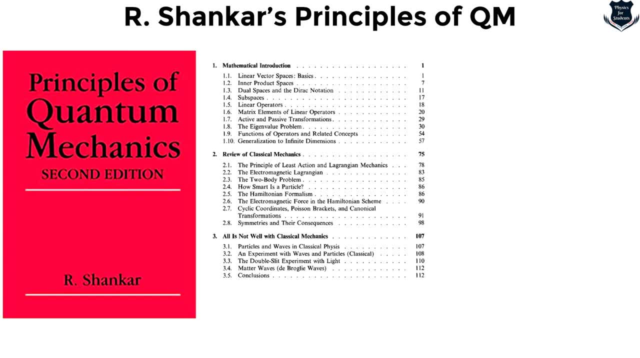 Linear vector spaces Everything. Then it reviews the classical mechanics. You see how Professor Shankar beautifully has done that: He is reviewing the classical mechanics, That is, the Lagrangian, The electromagnetic Lagrangian, The Hamiltonian formalism, etc. 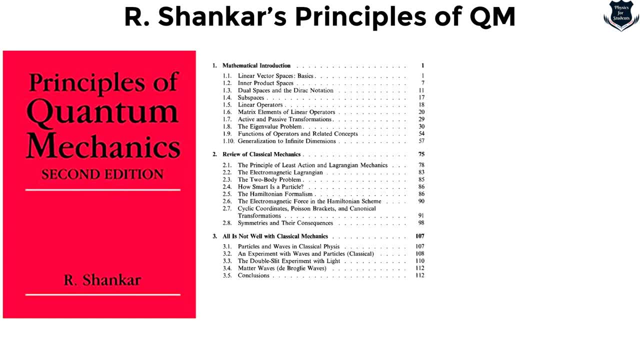 Why Professor Shankar is reviewing, Because it is always better to first review over the classical mechanics And then jump into the modern mathematics and physics of quantum mechanics. Then he writes this: all is not well with classical mechanics. Obviously, all is not well. 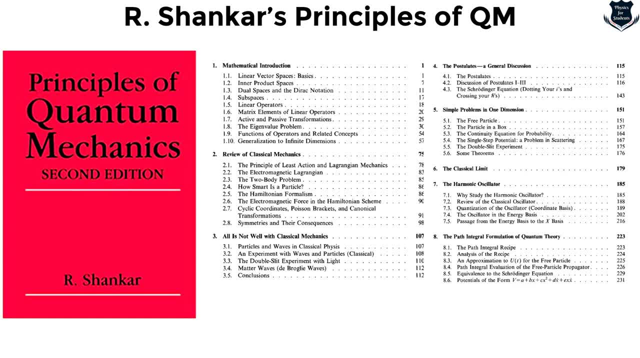 Because the double slit experiment actually shows the wave particle duality. Then he starts with the postulates. The postulates: discussion of postulates 1, 2 and 3.. Again, it is very systematic because without understanding mathematics, Without reviewing the classical mechanics, 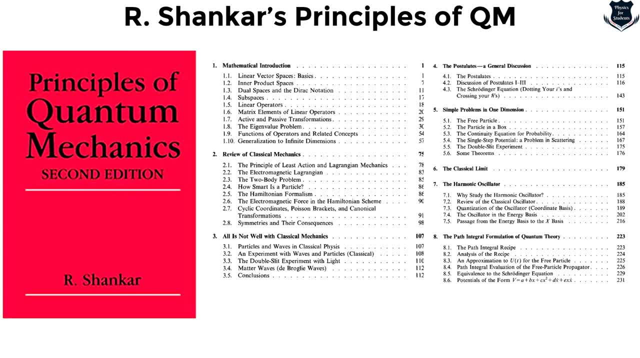 Without understanding the limitation And without the basic principle, that is, the postulates, How can you go into quantum mechanics? Then he takes up into a simple problem in one dimension, The classical limit, The harmonic oscillator, The path, integral formation of quantum theory and so on. 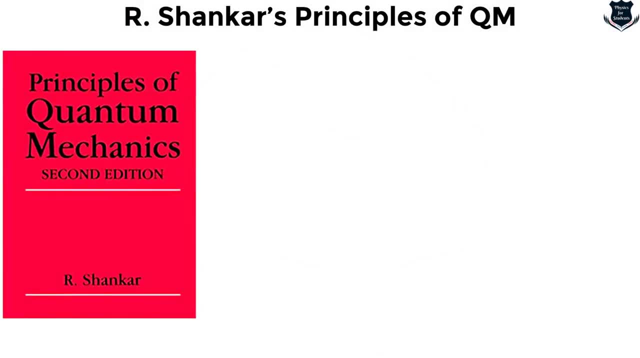 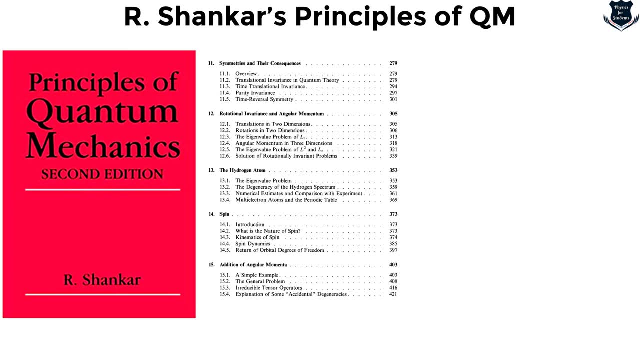 So what I wanted to tell you is that you see that the way the book has been organized Shows that this book will be just amazing. Symmetries and their consequences are defined. Hydrogen atom- again the eigen value problem Spin. So more or less, if you see the books by great authors and professors, 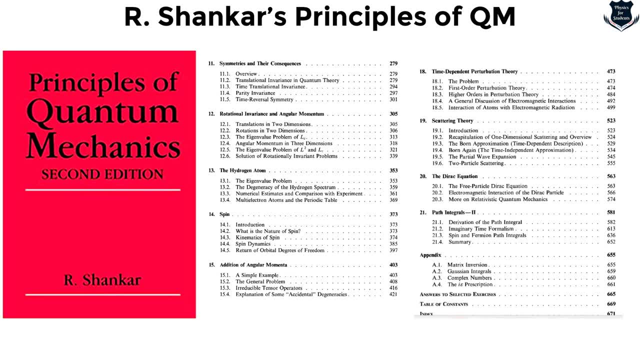 The organization itself depicts that the book will be fine. He then goes into time: dependent perturbation theory, Scattering theory, Dirac equation, The path integrals part 2. That is the spin and the fermion path integrals. And then he finally proves and concludes. 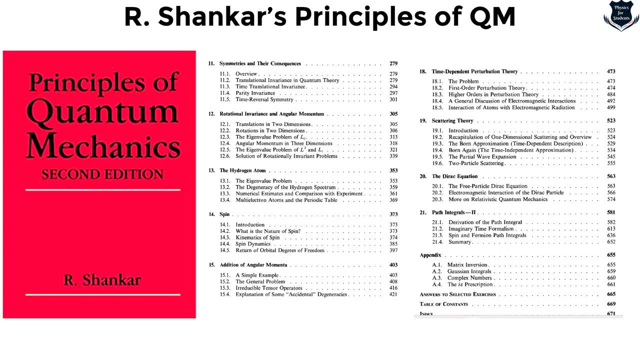 With the appendices. So this is also a great book by R Shankar. You know, if you just follow line by line, Chapter by chapter, Without skipping any part of it, I think you are done. You are done with quantum mechanics. 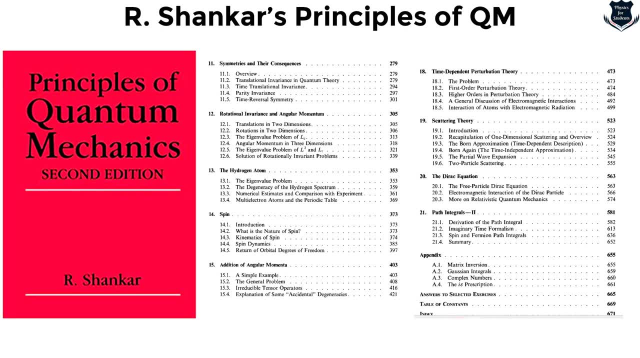 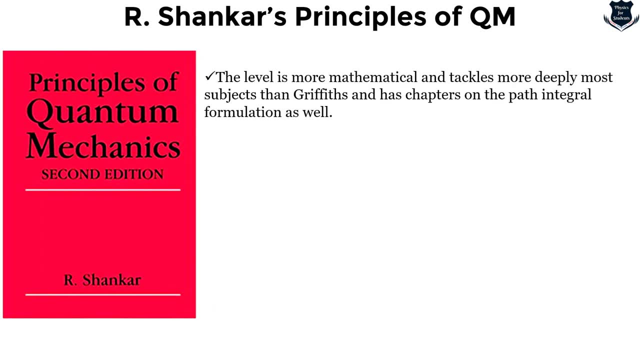 Because you know the basics, The mathematics, The limitation, The postulates, And then you go into the physics. So I think that would be great. So my review would be that this level of, The level of, is more mathematical And it tackles things much better than Griffith's book. 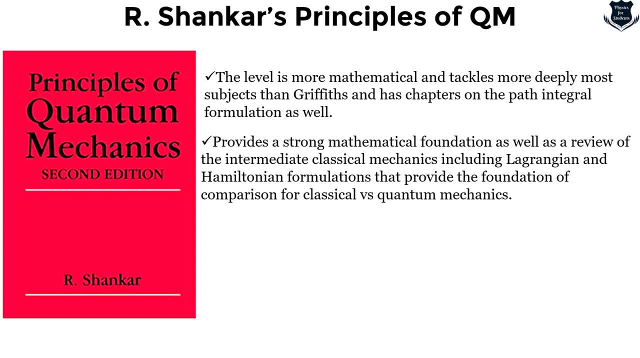 Right. It provides a strong mathematical formulation, Which I was telling That, with a review of the intermediate classical mechanics Including Lagrangian, Hamiltonian, Etc. And it contains two big chapters, Remember: One is the mathematical method And then the classical mechanics. 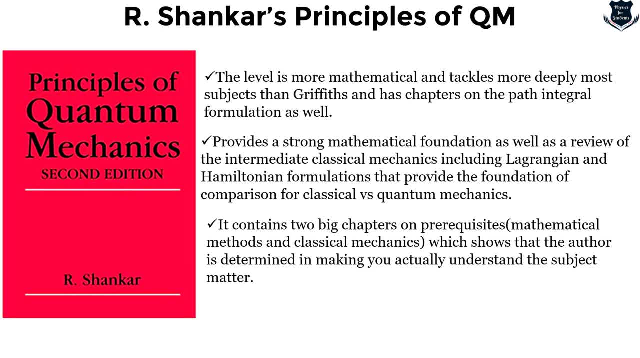 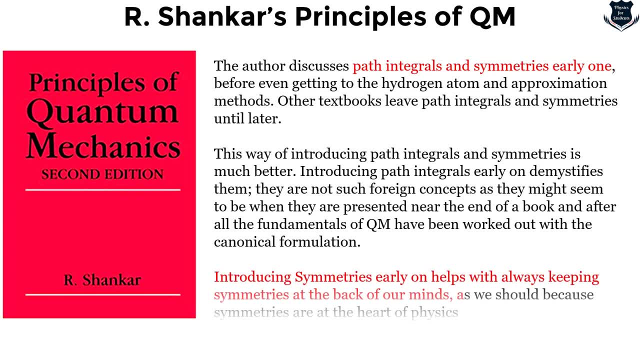 Which basically makes the foundation very strong Before you go into quantum mechanics. It also I would say the author discusses the path integral And symmetries early on, Before getting Even in getting to hydrogen atom, Because other books I have seen. 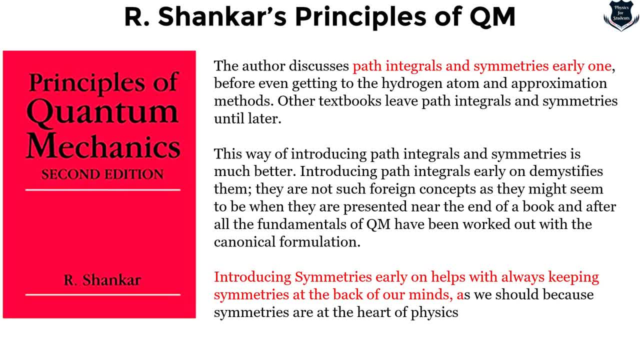 That they leave the path integral Much later. But this is good, That you learn the path integral symmetries earlier And then go Into the hydrogen atom approximation, And this way Of introducing path integral Is much better, Because introducing path integral 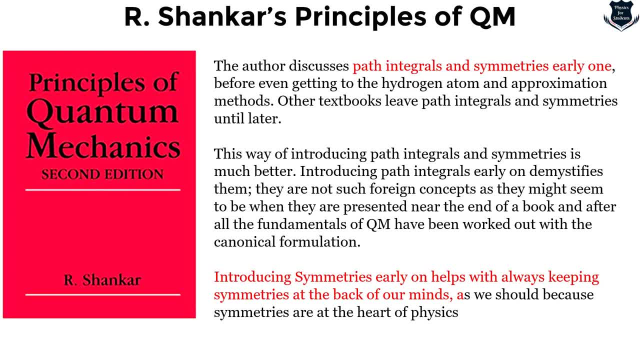 Demystifies some of the mysteries And when they are represented At the end of the book. You have already done with that. Also, Introducing symmetries Helps to keep your mind At the back, Because these are Basically. 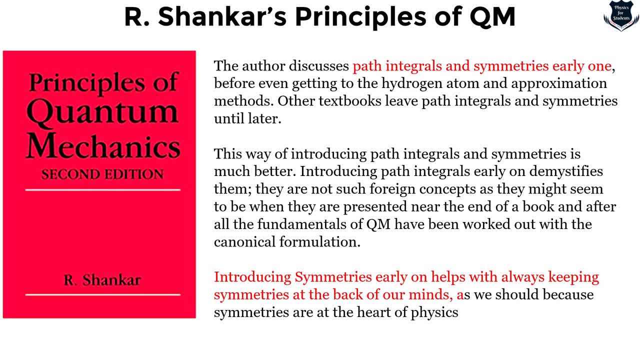 The core concepts And the heart of the book That you have already done with that. Also, Introducing symmetries Helps to keep your mind At the back, Because these are Basically The core concepts And the heart of the physics. 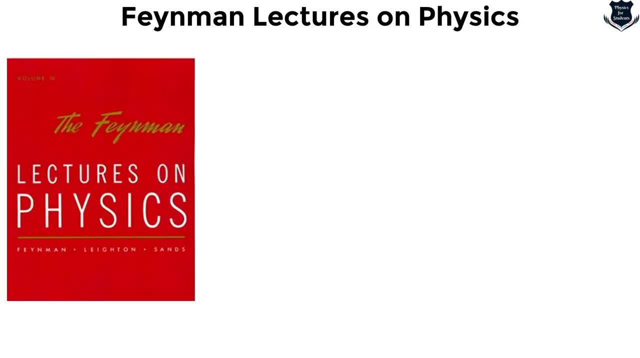 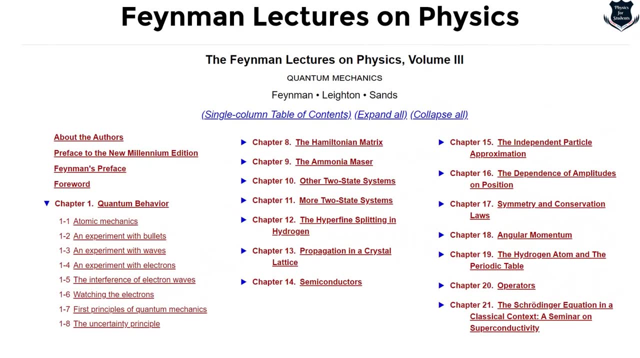 Lies in that. Okay, I think this book Requires no introduction. That is called Feynman lectures And physics. 88 percent Has given a five star, And the good part Is that This book Is already available. 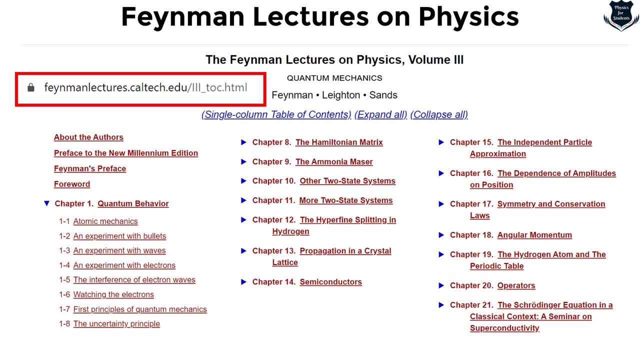 Online. I mean to say The lecture notes Is online, So I have given it In block. Feynmanlectures- caltekedu. So you can just go to Caltech's You know Website And you can just. 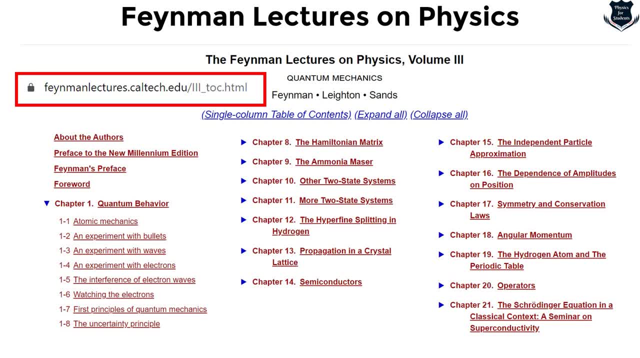 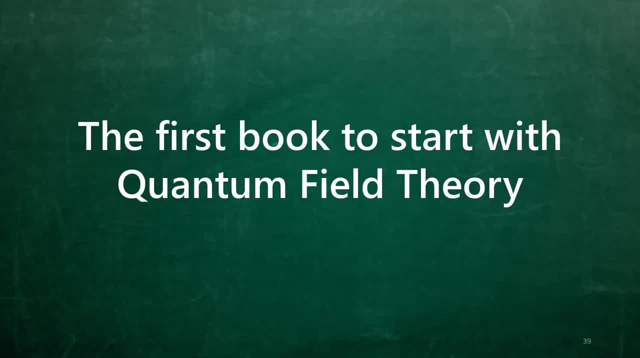 Read, Download and clear with 1,, 2,, 3 and further volumes. So all the physics, starting from classical mechanics to classical mechanics, is given. Now that we have done with the quantum mechanics, obviously we have to first start dealing with what we call the first book, to start with quantum field theory. 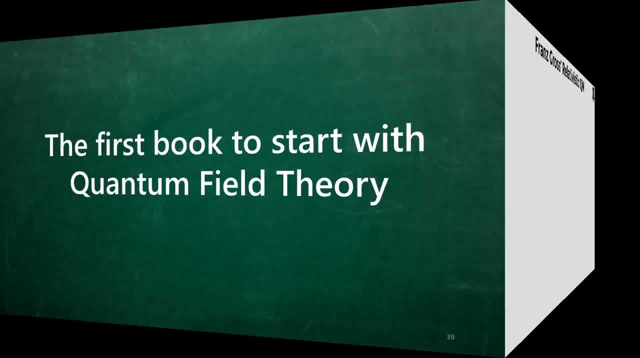 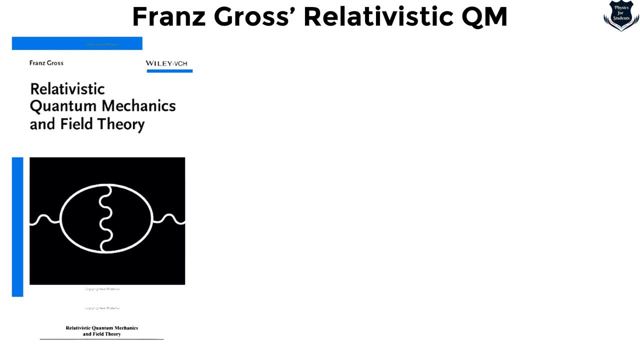 and to your surprise this book is not about directly quantum field theory, but this is what we call Franz Gross, relativistic quantum mechanics and field theory. Obviously, relativistic quantum mechanics means quantum field theory, but this book again builds up on the quantum mechanics, uses the relativistic equations and then goes into field theory. So here is the kind of a review. 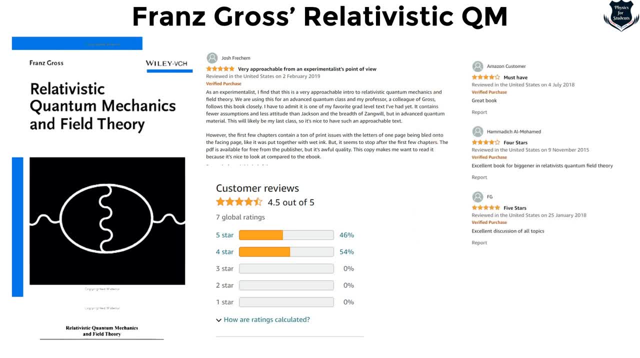 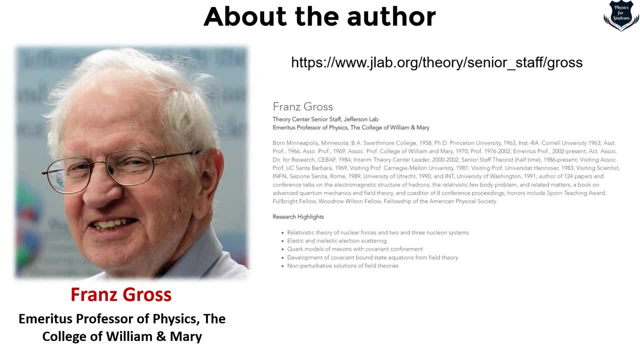 as an experiment. I find this is very approachable. few people say must have four stars: excellent book, excellent discussion, all of the topics. If you really want to know about professor Franz Gross, you can go to this website, and he is a emeritus professor of physics at the college of William. 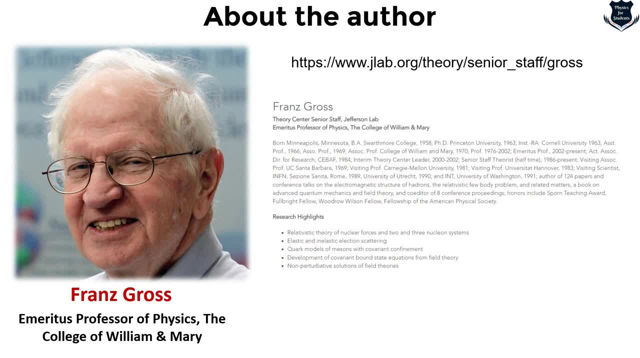 and Mary and you can go to his website and you can go to his website and you can go to his website and just read about it. I always feel that before learning the book or before going out with the book, it is important to know who is the author, so that the credentials and other style of reading is also 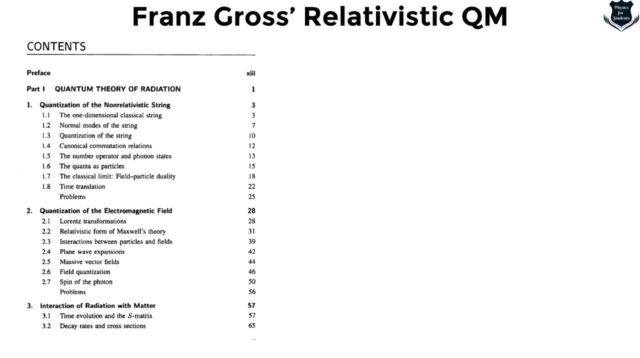 being concerned. So Franz Gross, relativistic quantum mechanics. it starts with the quantum theory of radiation quantization and run, relativistic string. then it goes into electromagnetic field interaction of radiation. Most importantly, part two starts with the Klein-Gordon equation, which is the first step in order for the unification. So you see he has done the 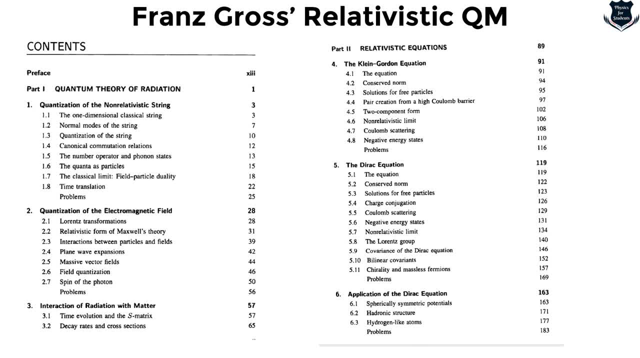 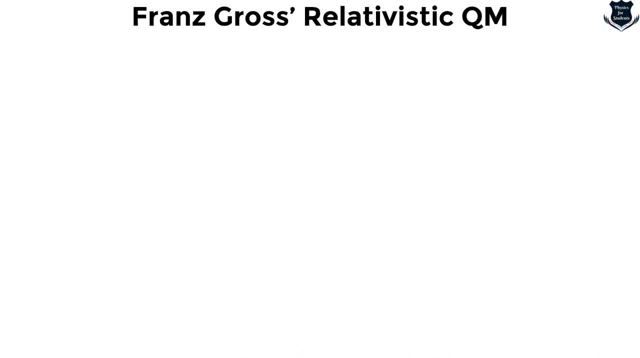 two component form, non-relativistic limit then. then you have dealt with the Dirac equation, which contains the Coulomb scattering negative energy states, application of the Dirac equation and so on. Further I can say that this is. it also contains second quantization, which is very 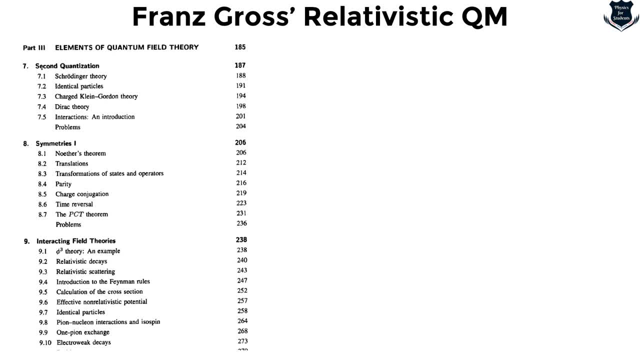 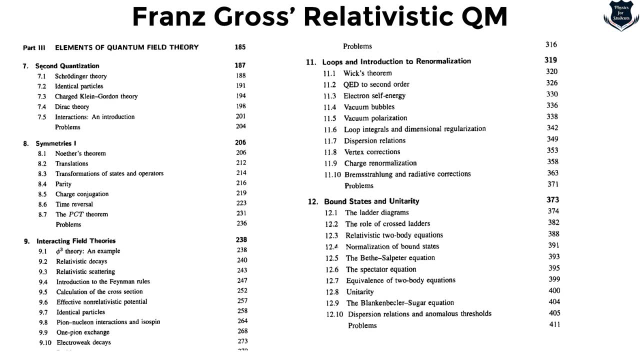 important: the Noether's theorem, as I was telling that you need to learn Noether's theorem, that relativistic decays, introduction to Feynman rules, loops and introduction of renormalization, vacuum polarization, everything I mean to say the relativistic decays, introduction to Feynman rules, 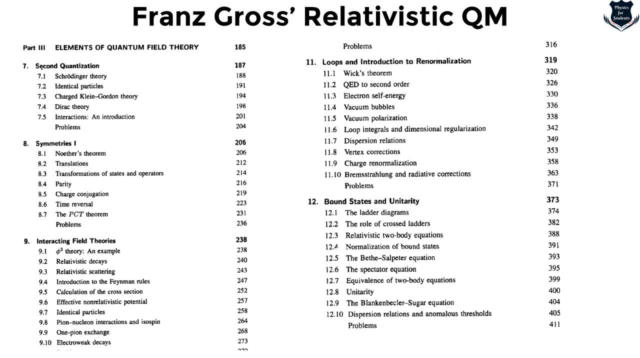 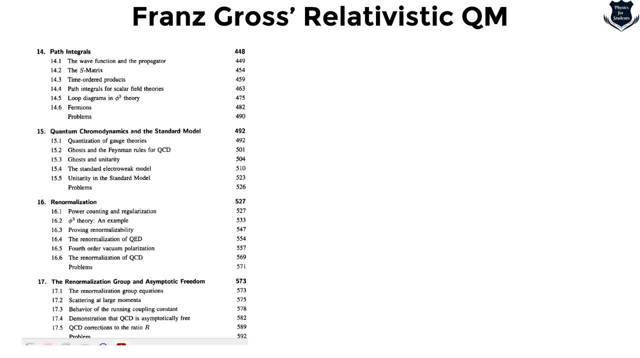 loops and introduction of renormalization, vacuum polarization, everything, I mean to say the relativistic part of quantum field, quantum mechanics, whatever the topics, whatever the things are required, it is included in this book. Finally, he concludes with this path integral, then renormalization and then the appendix. 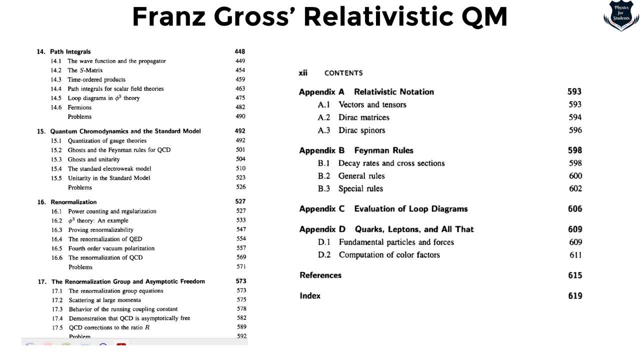 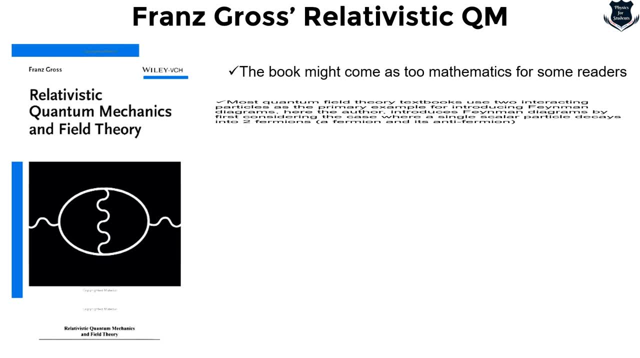 the, which includes vector and tensor, Dirac matrices and Dirac spinors. Now my take of this book would be: initially, this book looks very highly mathematical and some readers might find it difficult, but the important part is that you see that most of the quantum field theory books 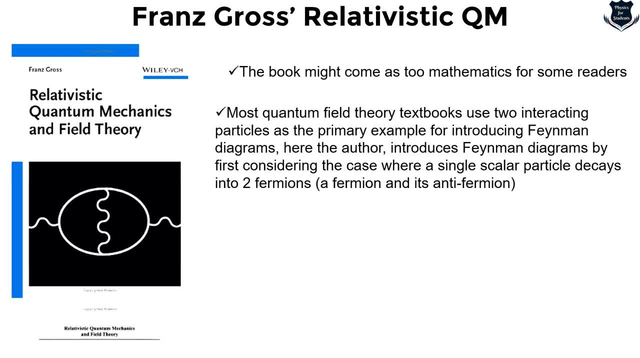 You're going to explain. you know find men diagram they introduces, basically, you know, the single, the two, two fermions apart. but here, as a primary Example for introducing finite diagram, professor Gross introduced at the single scalar particles instead of to for me on. So what happens things? 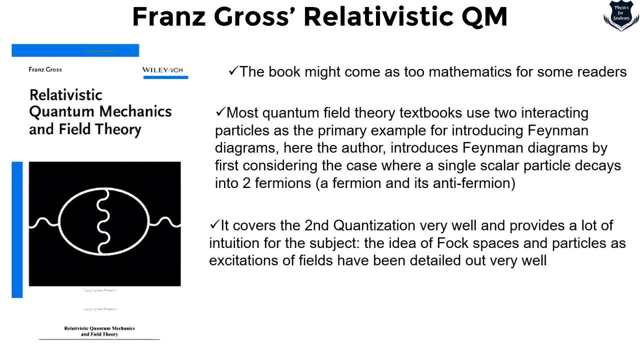 now Maya becomes much easier. the secant quantization, the fox places, et cetera, very much clearly, you know, covered up. So there is absolutely no problem on that. but if I just let me'll just give it a little more detail, so what happens is there is a single scalar particles instead of two fermions. so what happens, things becomes much easier. the second quantization, the fox places, etc. very much clearly covered up, so there is absolutely no problem on that. So there is absolutely no problem on that. 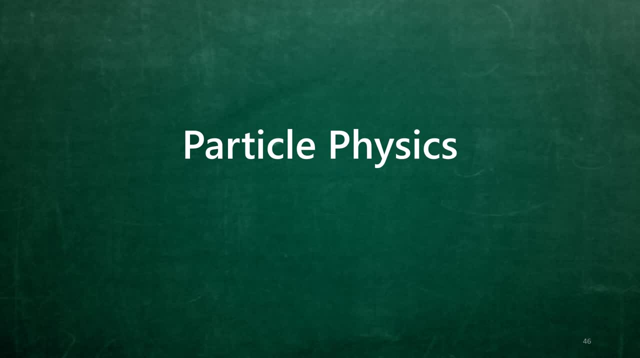 so we now come to what we call that. what, other than the things required? we have understood quantum physics, we have understood the mathematics, the one thing which is lacking, which is called a basic idea and introduction to particle physics, because quantum mechanics and even quantum field theory is all about particles, their interaction. so basic knowledge and introductory knowledge of 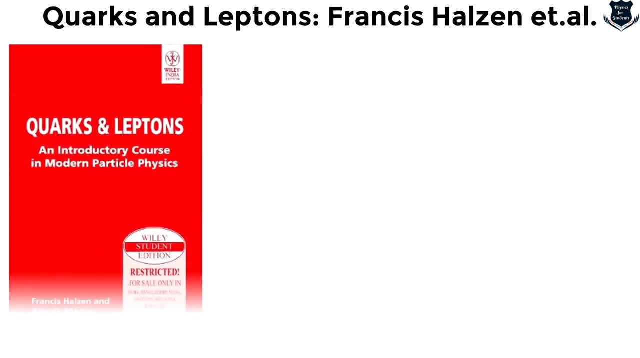 particle physics is something which is required, and i would recommend this book, quarks and leptons, which is an introductory course of modern particle physics by francis halzen and alan d martin. this has got a kind of a rating of 65 percent of five star, but this is just an amazing book. let me show. 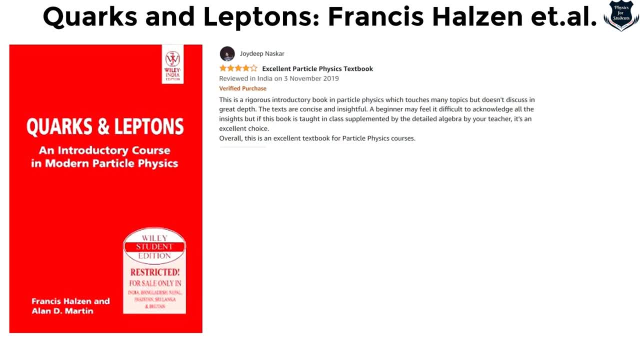 you the table of contents before that. here is a quick review of those. this is a rigorous introductory book in particle physics. overall this is an excellent book. some says this book gives a precise and to the point explanation of the particle physics concept. nice book, very good introductory. 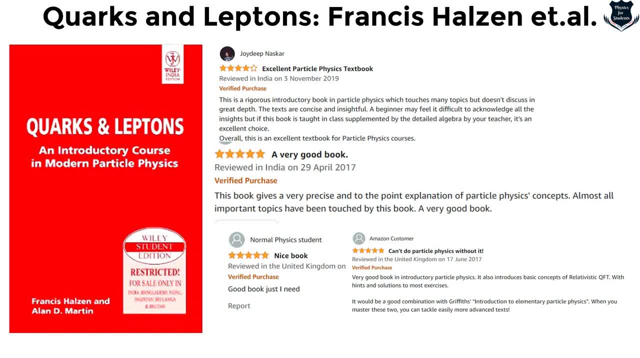 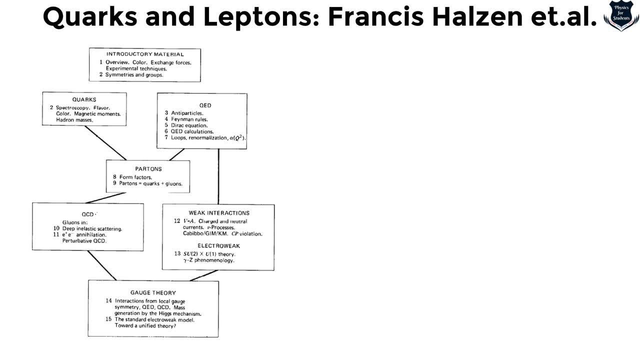 physics. so, more or less, you can see that this is a very good book and i would recommend it to you. what you can see that from these snapshots that this is a very book book in terms of, uh, understanding the basics of particle physics. so let us see what are the table of contents. before that, the 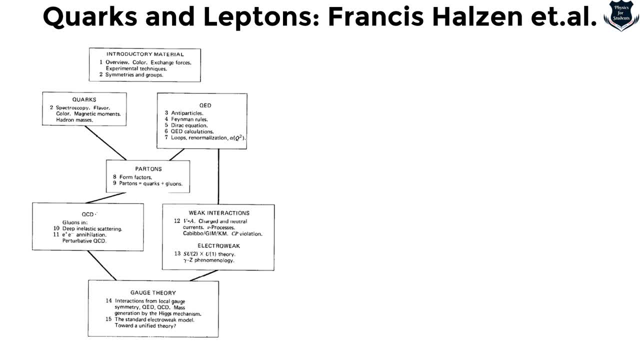 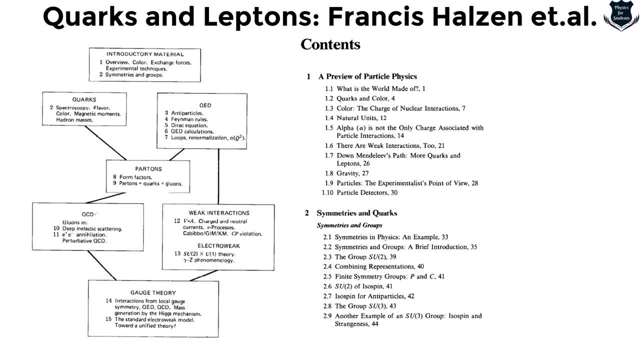 it starts with gravity, the particle detector, so you get a basic idea that what the uh, particle physics and what, what it is all about. so you can get a fair kind of an idea. then it starts with symmetries and quarks, symmetries in physics. what are symmetries in physics as a whole? 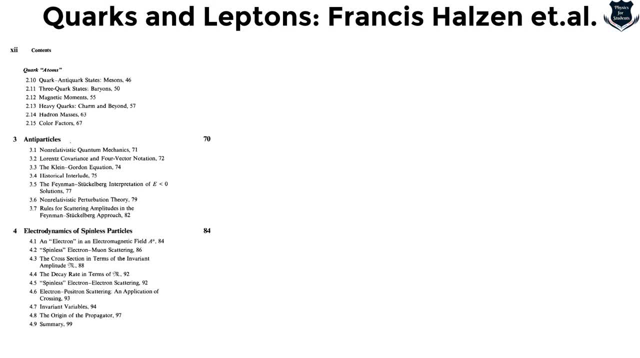 uh. we go to the next page which shows uh, quarks, atoms, anti-particles, which includes again the klein gordon equation, the electrodynamics of spin less particles. it is good point to start with spin less particles so that with spin less particles it becomes a needed field for interaction with. 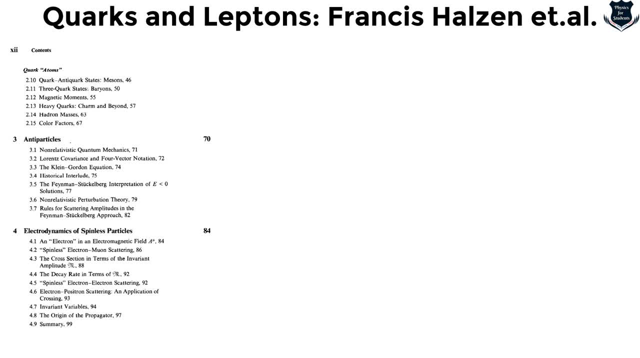 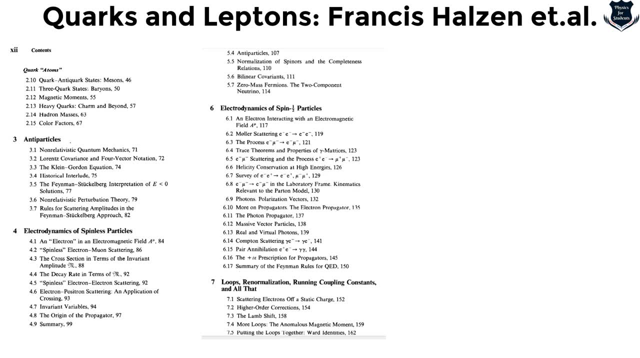 spin particles, the chirality, etc. becomes too much complex. so it starts with the decay rate, electron positron scattering, invariant variables and so on, and you can see that electrodynamics of spin particles concerning photons, polarizations, vectors, photon propagator, real and virtual photons, competence, scattering, pair analysis and everything, whatever it is concerned, related what you need to. 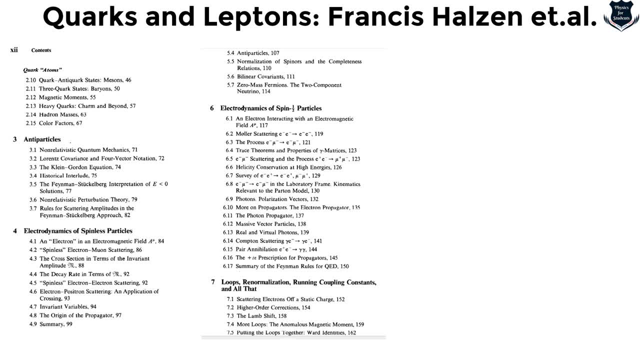 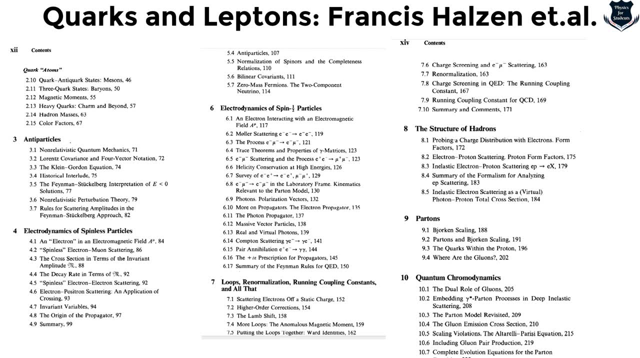 know about particle physics, not going into too much details but at least explaining the basic concept part- that is already done- the structure of hadrons, including the probing e charge distribution, then the pair, the patterns, which includes the quarks within the proton, and a part of quantum chromodynamics, although again it's a very complex and a lot of mathematics required. 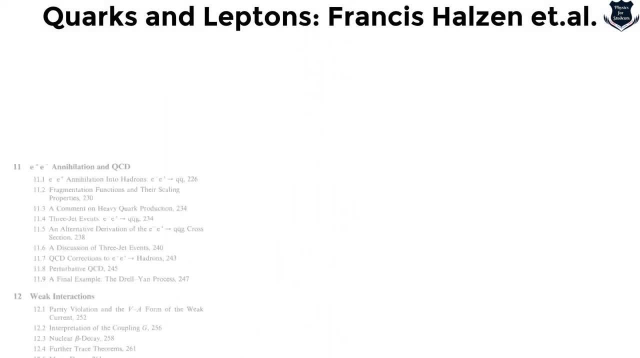 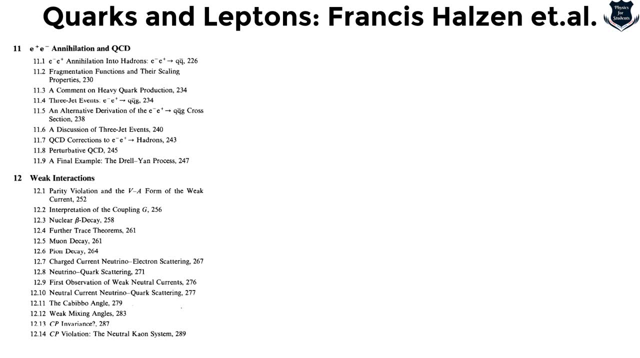 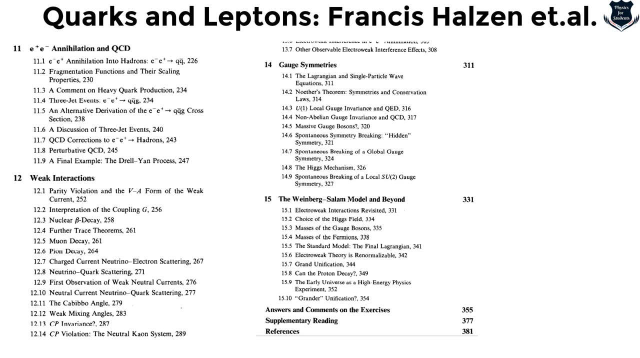 but it covers comprehensively what is called the quantum chromodynamics. then it starts with the annihilator and the- you know, constructive operators: a weak interaction, pi and decay- these things are already being covered. and then it starts with gauge symmetries. again no hs theorem symmetries. 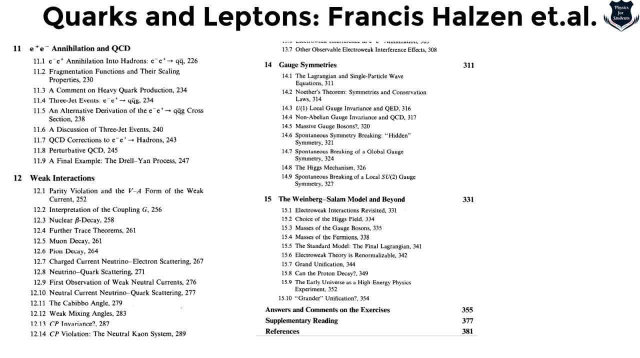 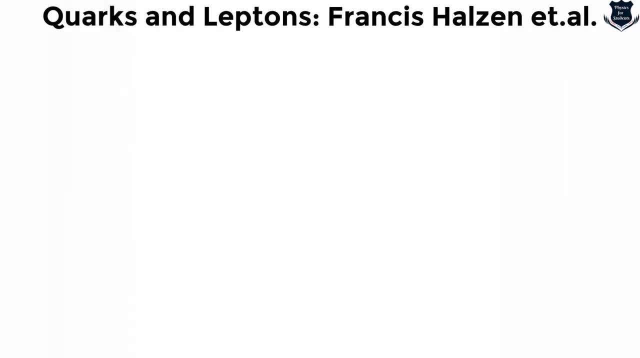 and conservation, weinberg abdul salam model. this is again very important. what we called is that? uh yeah, it is an electroweak theory, so all these things are being covered. so my review for this book, quarks and leptons, would be great. these are few of the you know diagrams. you see, these are. 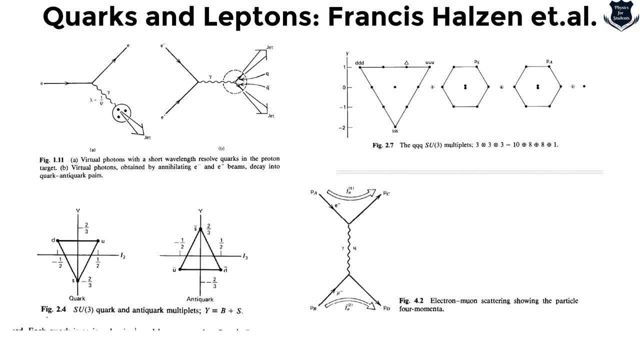 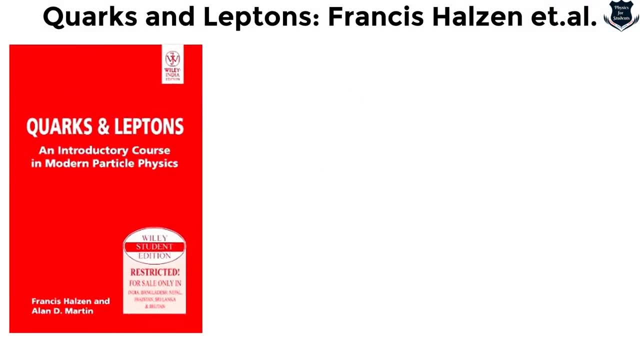 beautiful diagrams because particle physics all about diagrams the annihilation particles coming in. so these are the few of the diagrams which explains things quite clearly. so my take would be: it is a very good book as far as the introduction of particle physics is concerned. it gives you a